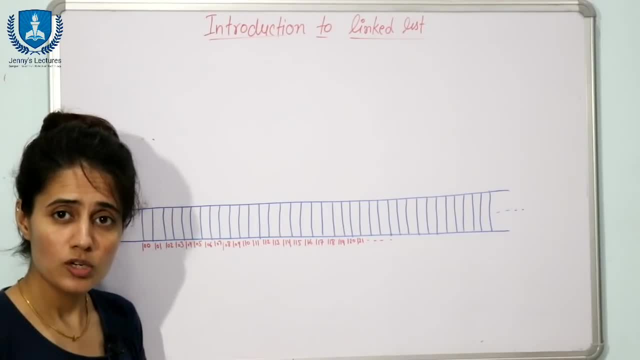 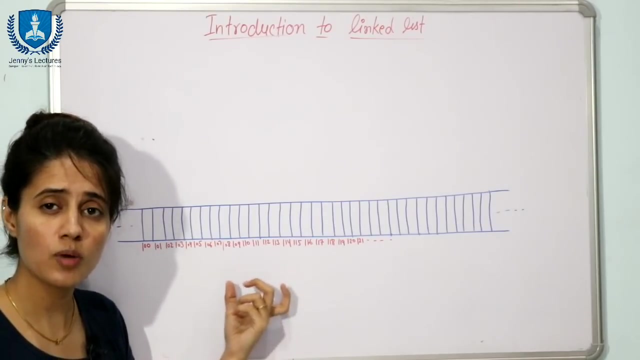 102 like this. See, this memory is very crucial resource in our system. We don't have unlimited memory in our computer system. Fine, So it is a responsibility of a memory manager to manage this resource, to manage the memory, to which process memory is to be allocated, how much memory is to be allocated, which memory is free? which memory is allocated now like this? Fine, So memory manager is going to take care of this thing. Fine, Now suppose a programmer want some memory, in this case a programmer. 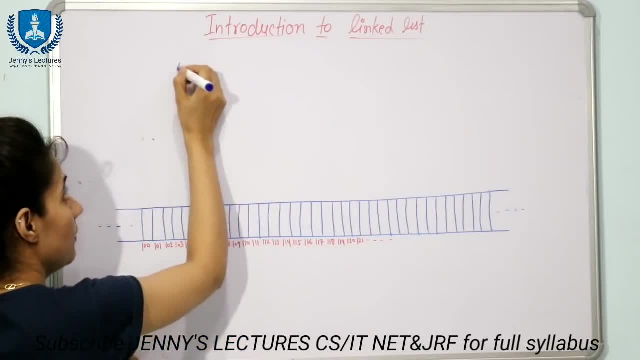 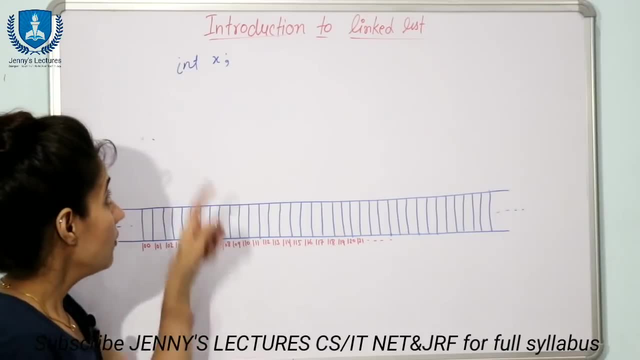 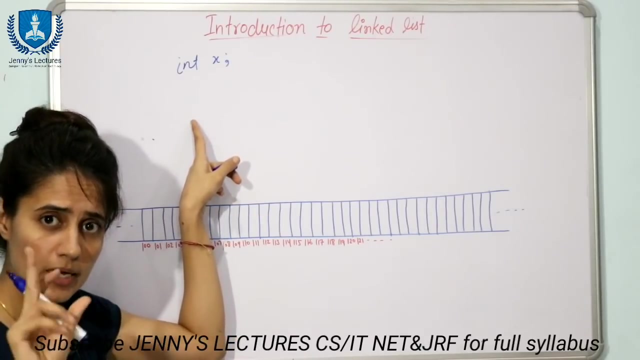 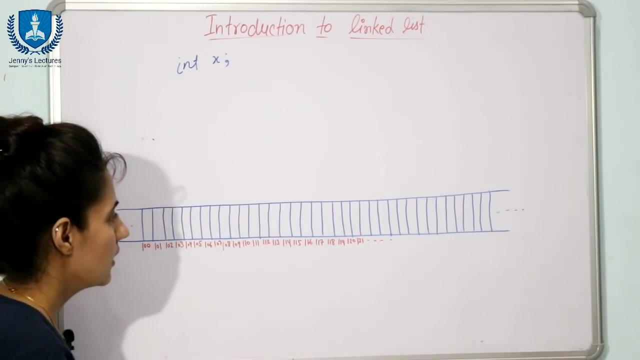 is writing a program and he is going to declare a variable like this. in suppose variable name is X, Fine. Now when, after declaring this variable, what happens? the memory manager will allocate how many bytes? 4 bytes for the synthesizer in typical compilers, Fine. So let us suppose memory manager allocated 4 bytes to this X and started from which location started from? Let us suppose this location. 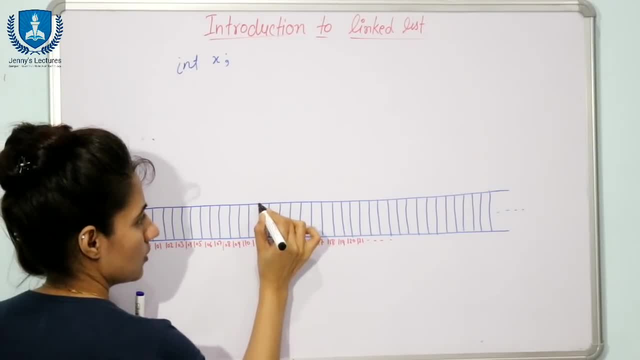 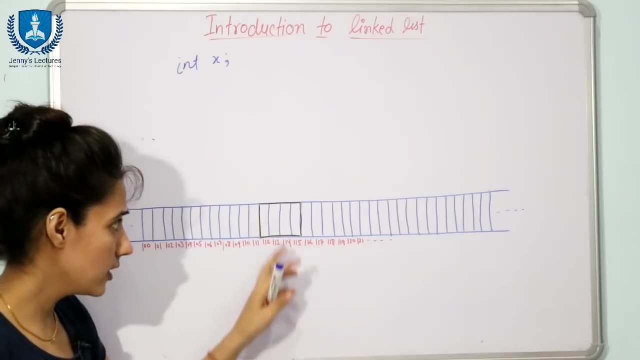 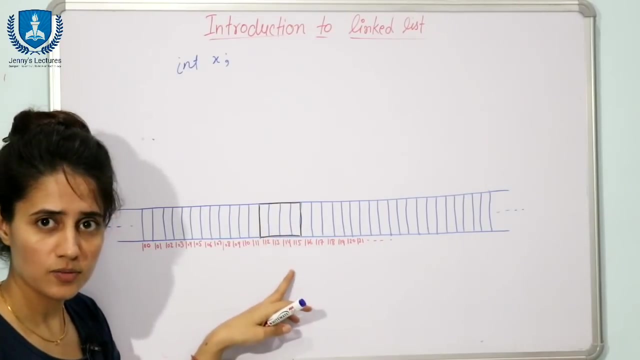 from 1, 1, 2, these 4 bytes. these 4 bytes has been allocated to this X and memory manager will tell the programmer that I have allocated to the memory which is started from 1, 1, 2, 1, 2, 3, 4 bytes. fine, and suppose he has entered some. he has. 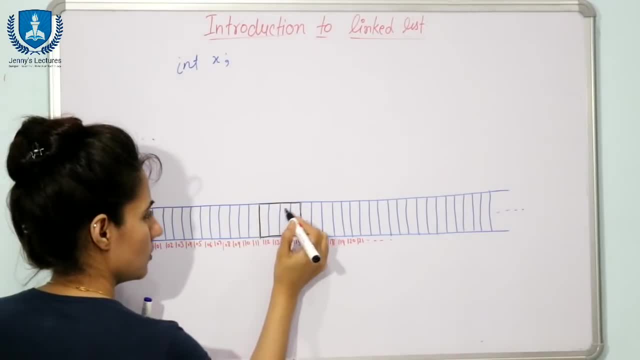 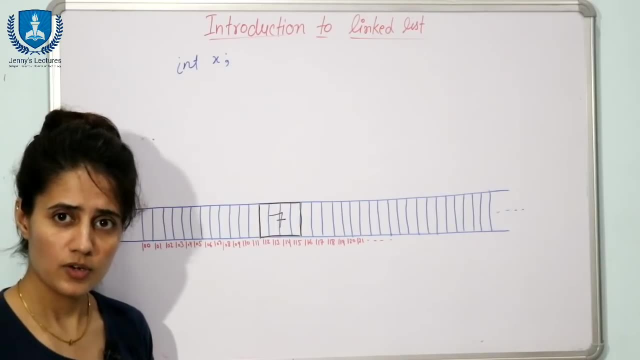 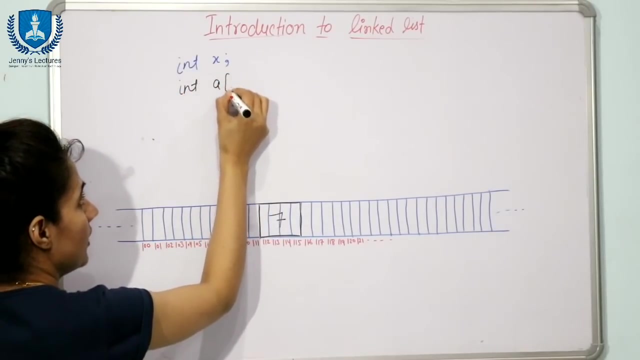 initialized at runtime, this X, and he can enter some integer value like 7. so now the programmer suppose we want to store three integers. fine, so we we have. we have read the concept of arrays, so how he will declare int. suppose array name is a and size is 3. so see, array is what it's: a collection of data, data items. which are of same data type. fine, so for 3 integers, for 3 values. the memory manager will allocate how many bytes. 3 into 4, that is 12 bytes. fine, and let that that 12 bytes would be 8.. consecutive continuous location: the integer, the values of the arrays are always stored in. 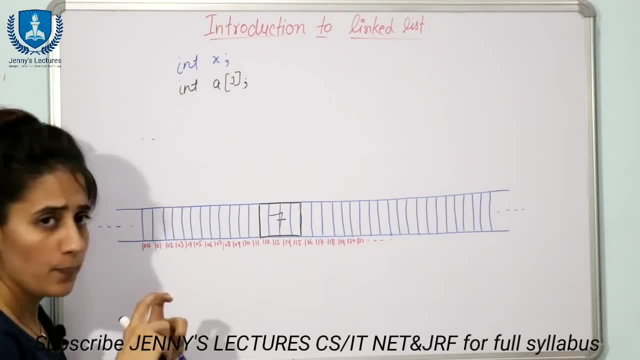 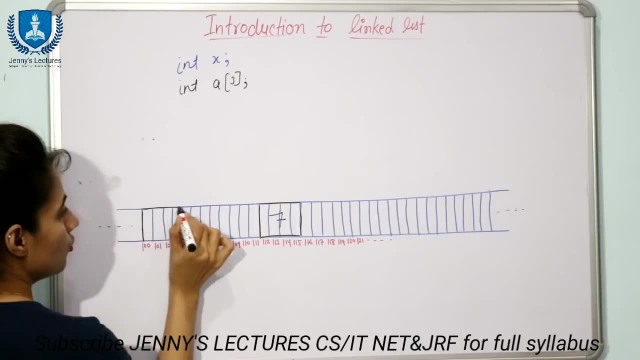 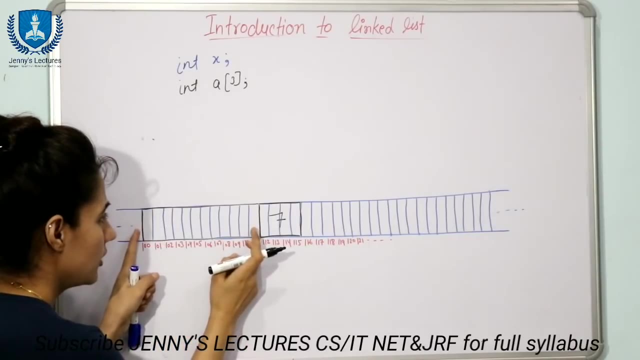 continuous locations. so let us suppose one complete block of 12 bytes has been allocated, suppose from 100 to from 100, to this: 1, 1, 1. this is free and memory manager has allocated the hello, has allocated this block to this array. so now programmer has entered three values here. 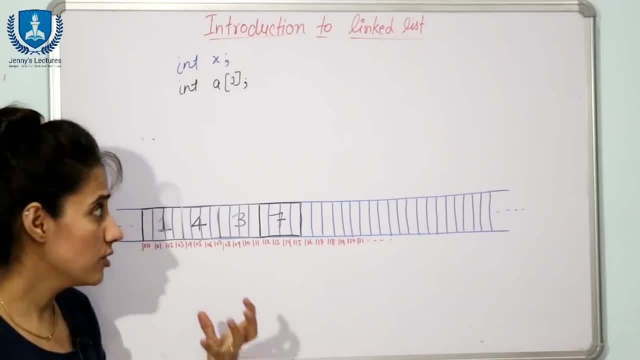 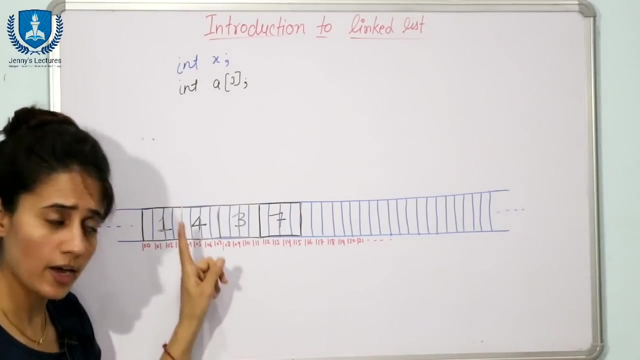 now the programmer wants to store one extra integer value, one extra value, and he wants to extend this array size. now he will ask, through the many memory manager, that i want to store one extra value. can i extend? can you extend the size? and i want to extend the same block. i want to extend the. 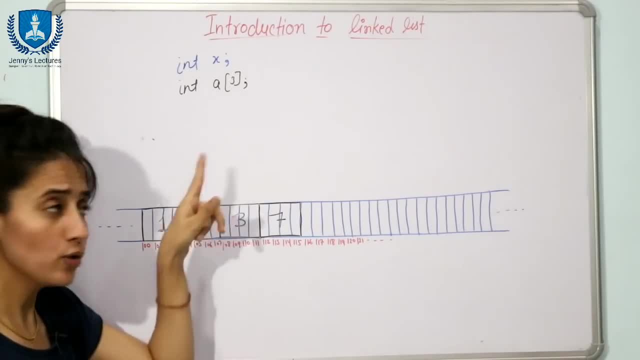 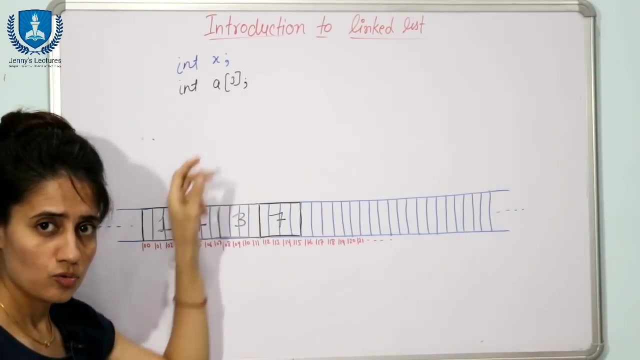 size of the array. i'm not going to declare another variable, i'm going to extend the size of the. i want size of array four now. now what memory manager will do see, because in in advance the programmer told that i want size for only three integers, so he has allocated 12 bytes. now what memory manager will say he will? 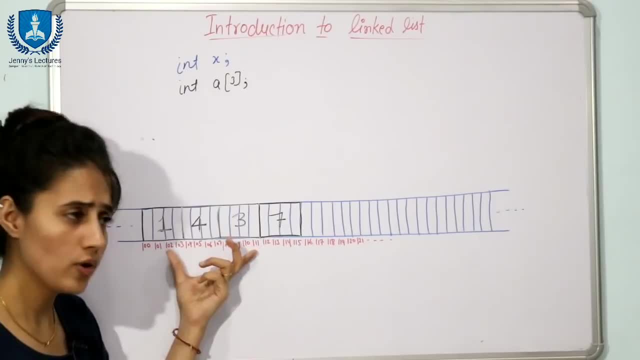 say: i cannot extend the size of your array because i have already allocated the that, that consecutive block, to some other variable. because at starting i didn't know that you are going to extend your array size. so now programmer will ask: what can i do now? i want array size 4.. so now? 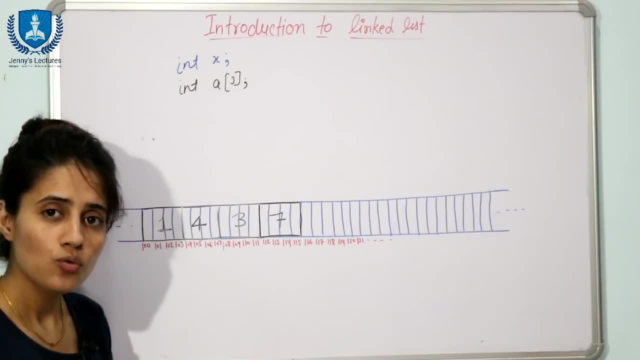 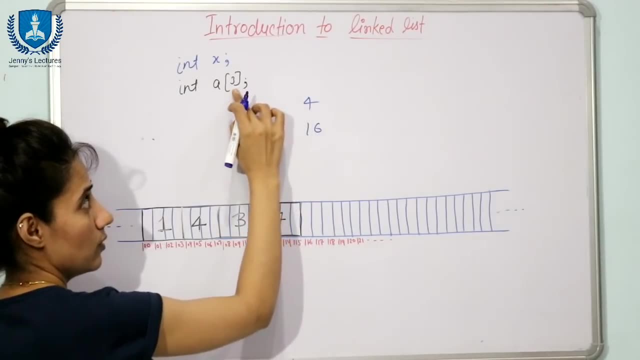 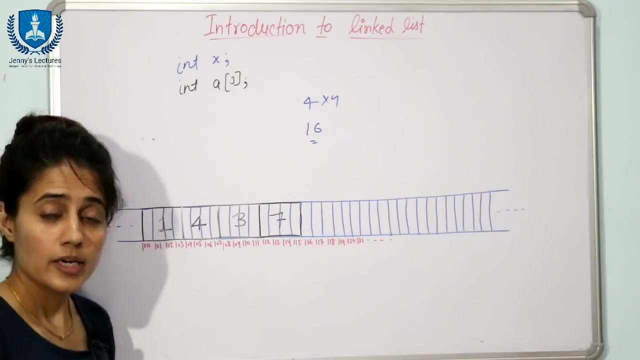 memory manager will say i can allocate you a fresh block of 16 bytes, because for 4- size of the array, how many bytes would be required? 4 into 4, that is 16. but i cannot extend this block now. what programmer will think? programmer will think that maybe in future i need to store 10 values. 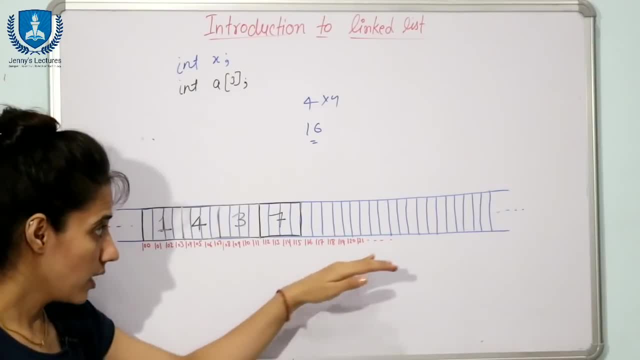 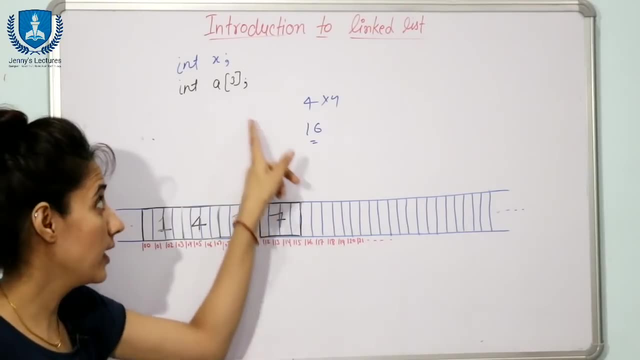 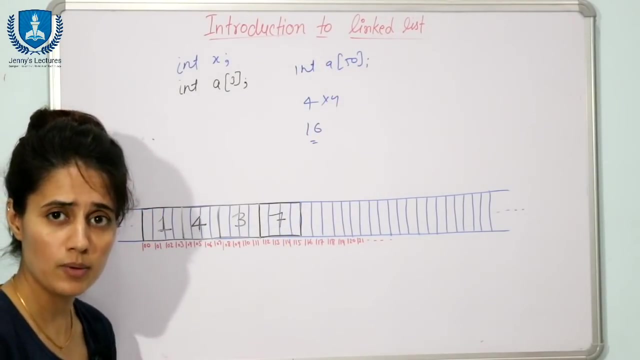 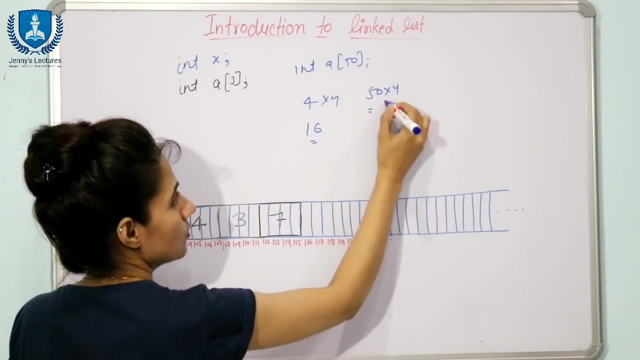 so it's starting. only i ask the memory manager to allocate me the size for 50 values for 50 elements that i want. my array size: 50 now int a and 50 maximum limit. now what memory manager will do? memory manager will locate how many bytes- 50 into 4, that is 200 bytes, a fresh block of 200 bytes. 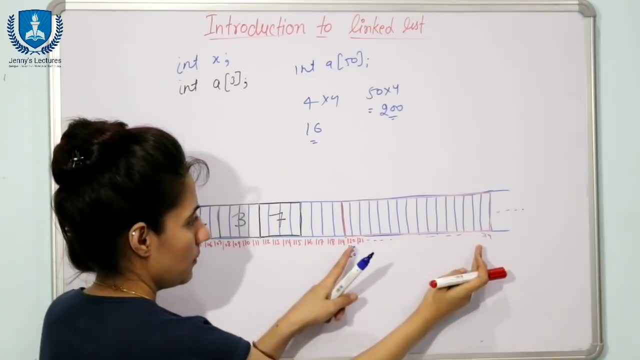 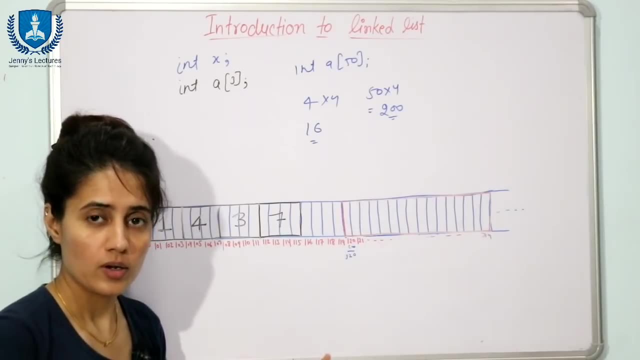 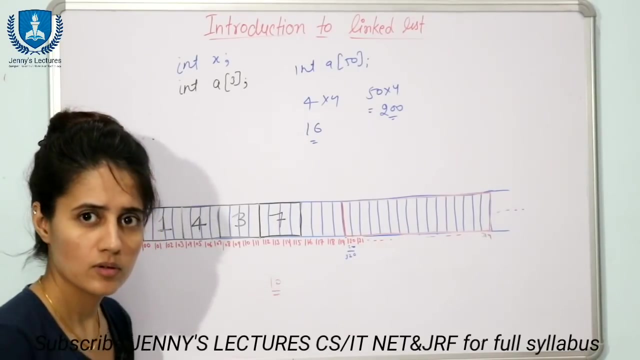 a consecutive locations. so these 200 bytes block is from- maybe you can say from 120 to this 319. address is 319, these blocks would be allocated to this one. but now suppose the programmer only needs to store maximum 10 elements. so this space is wasted now because he is going to use only how. 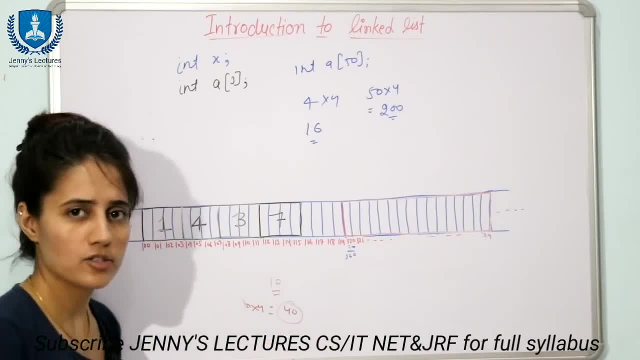 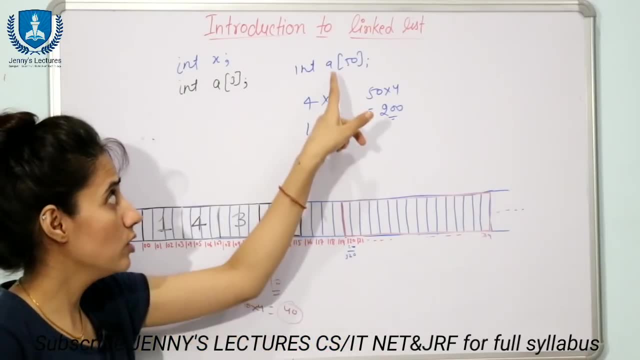 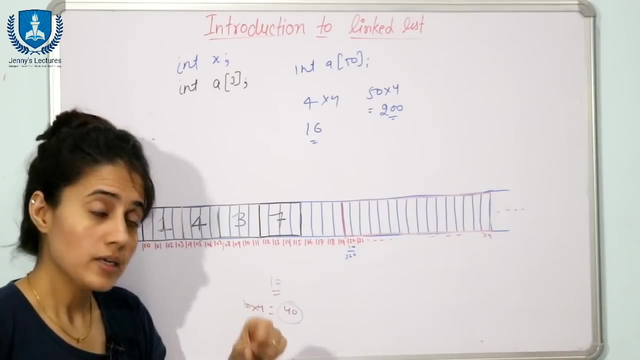 many bytes: 10 into 4, that is 40 bytes. he is going to use starting 40 bytes right and remaining memory. that memory has already been allocated to this array now, so memory is not free. the memory manager cannot allocate this free memory to another variable, but this programmer is not using that. 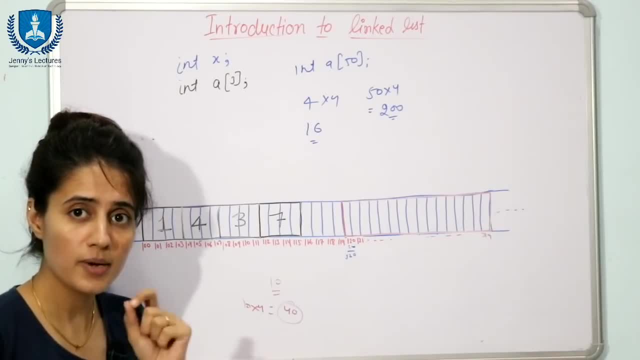 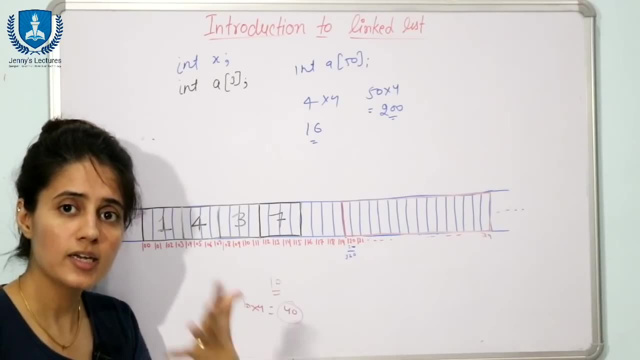 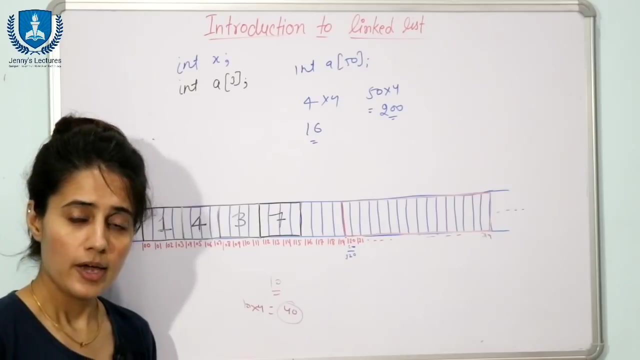 memory. so this is what wastage of memory. so this is a main drawback of n. because of the fixed size, because the programmer has to give fixed size of the array in advance at compile time. only because of this wastage of memory is there in case of arrays. fine, now what is the solution of the? 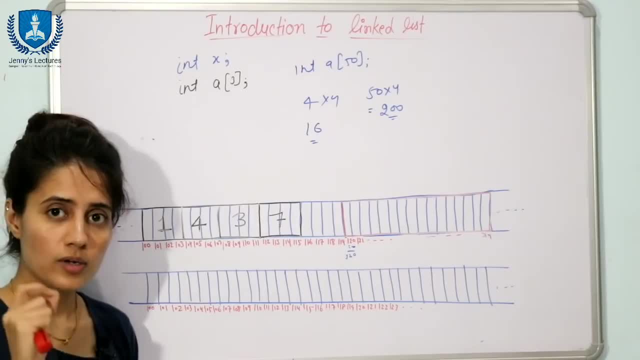 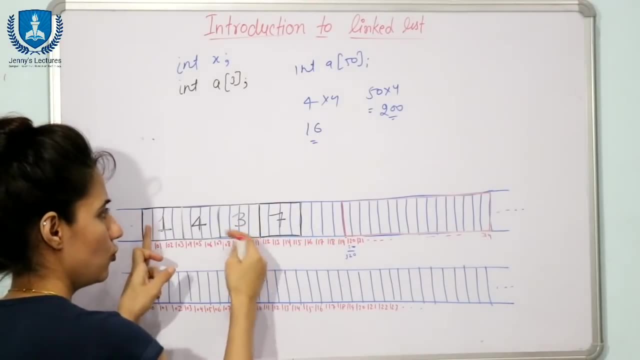 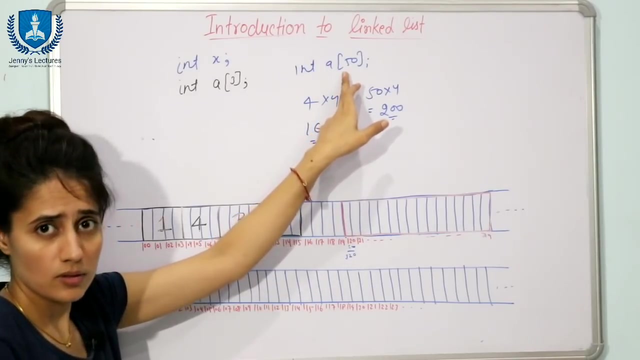 this problem. so now the solution of this problem is what linked list and here here see, if the memory manager has allocated these fresh block, then these values would be copied here only. so that would be a very tedious work to do and again suppose after some time, this, this, the programmer. 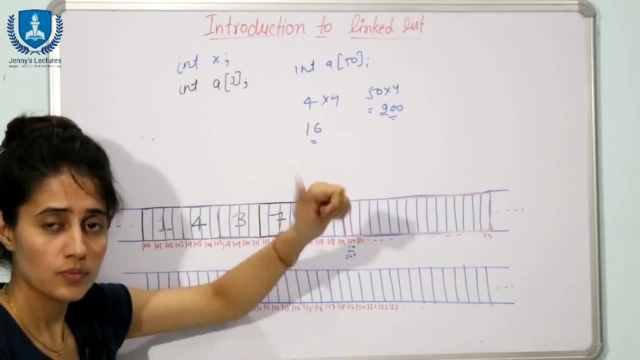 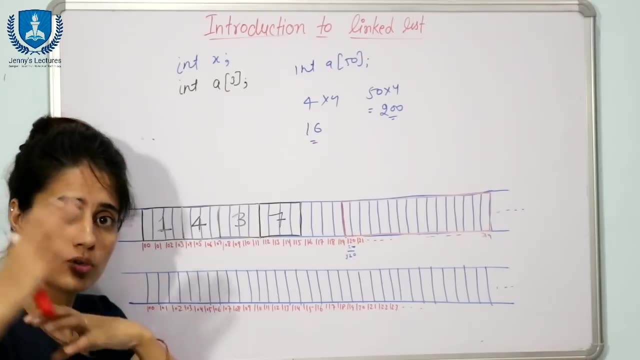 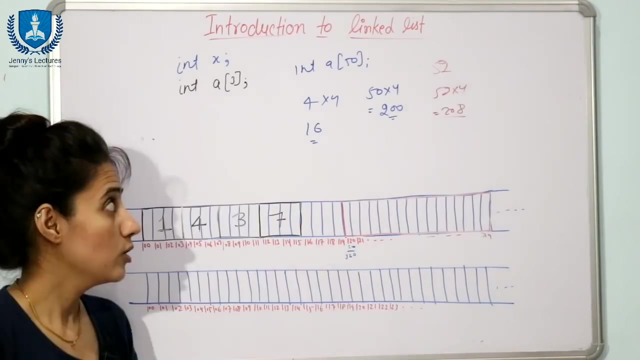 wants the size. programmer wants to store 52 elements. then again, programmer maybe is not able to extend the memory in some cases. then fresh a block of for 52 for 52 elements. how many bytes? 52 into 4.. so 208 bytes would be allocated. a new block of. 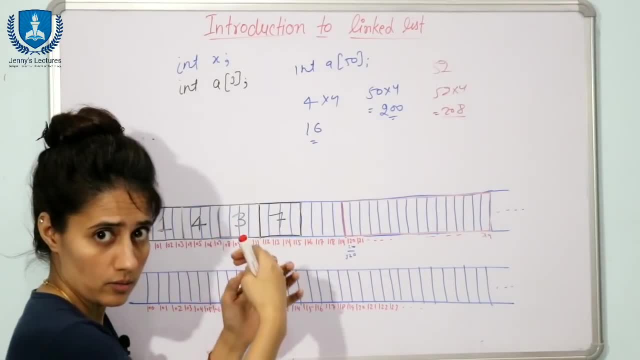 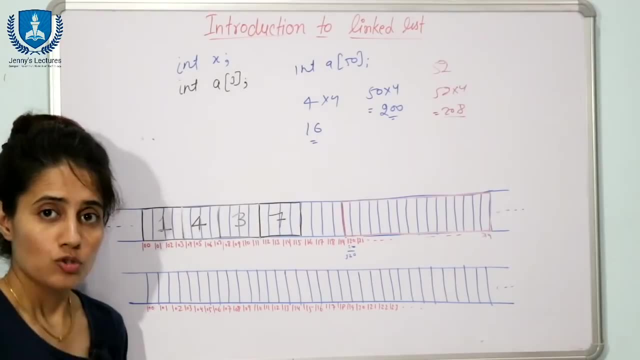 208 byte would be allocated and all the that elements of this previous array would be copied there. so that does very tedious work to do in arrays and the solution is what linked list. so linked list is also a collection of elements, see array. is what? also a collection of elements? 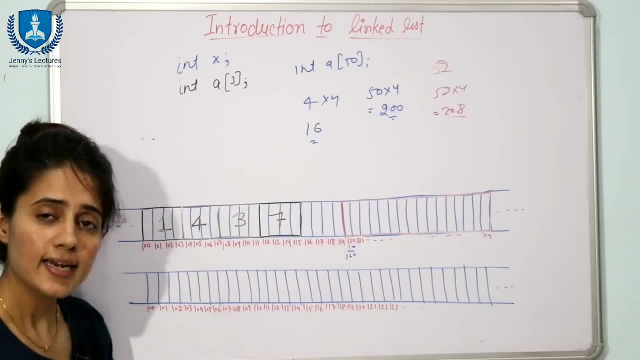 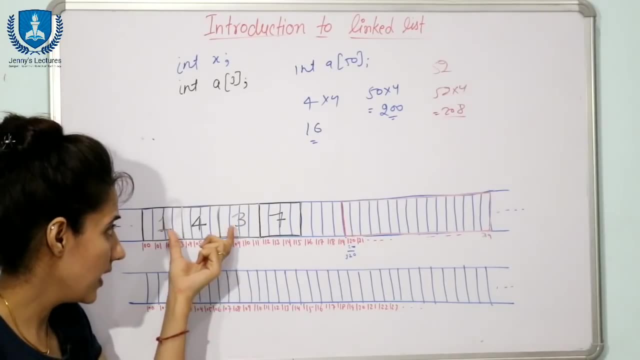 right, it is a collection of more than one data items. fine, linked list is also a collection of more than one data items, but the only difference is what in linked list- this, this data items are not stored in consecutive locations because this in array, these are stored in. 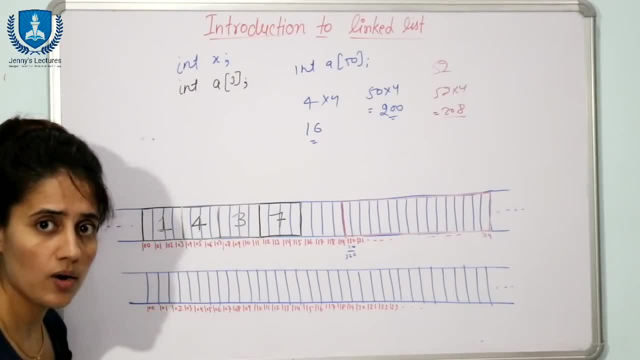 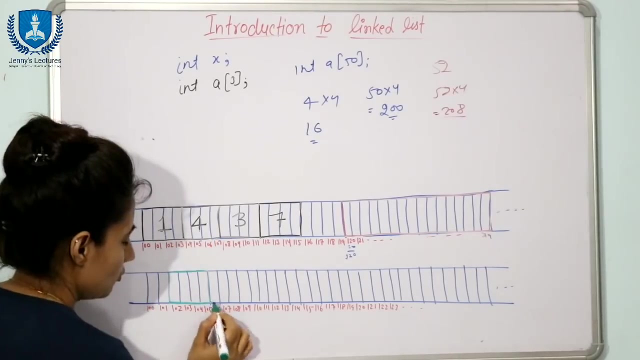 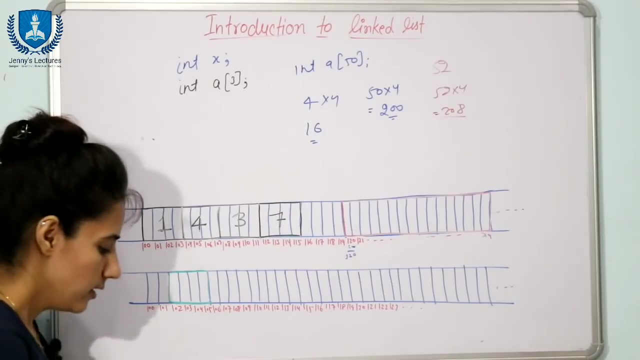 consecutive location, continuous location. fine, now how see if the programmer make a request for one element? he wants to store one element? fine now the memory manager suppose allocated and for integer value, four bytes. so suppose memory manager has allocated these four bytes right for the request of integer variable, and suppose he has stored some value that is. 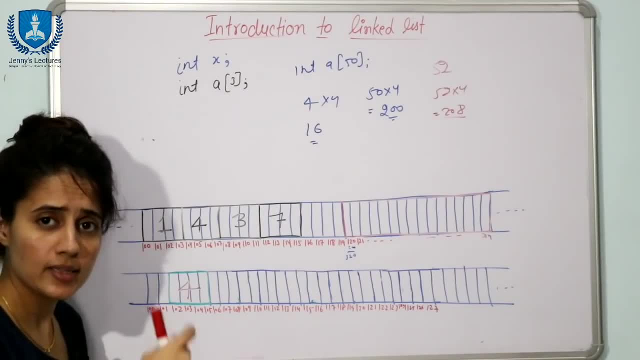 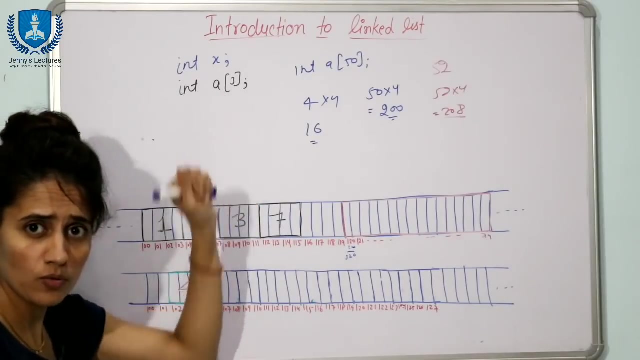 four here. after this suppose he has made another separate request for one variable, that is for storing an integer value. so again four bytes would be allocated. but it is not compulsory that that four bytes would be allocated consecutive to to this, because that is a separate request, that is not a request in form of array. so suppose now for next request, memory manager has allocated. 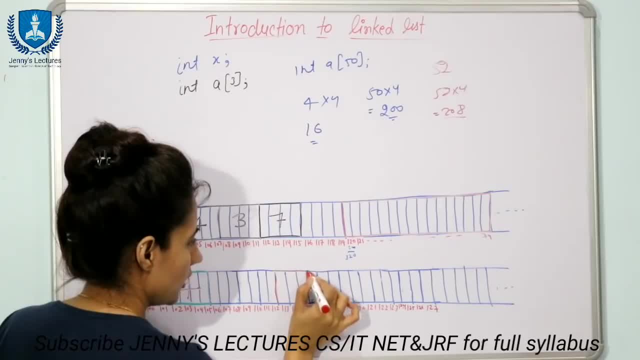 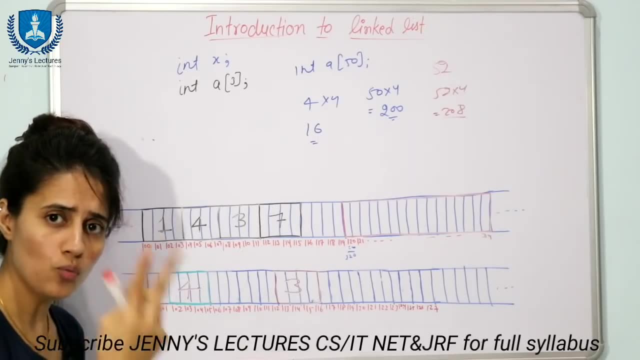 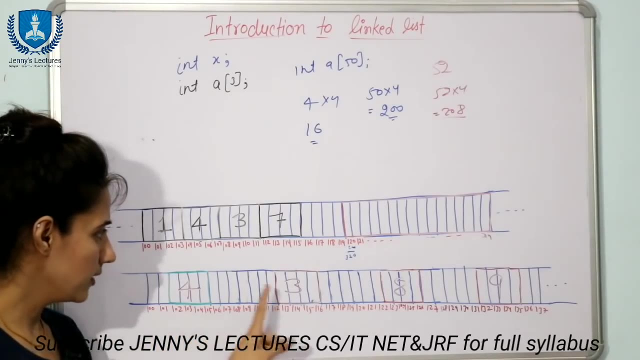 two more blocks from here, four bytes right, one, two, three and four, and he has stored here, suppose, three. fine, now again he has requested two more requests for inc for storing integer values. so now, this is how, for the four separate requests of for integer values, the memory manager has allocated: 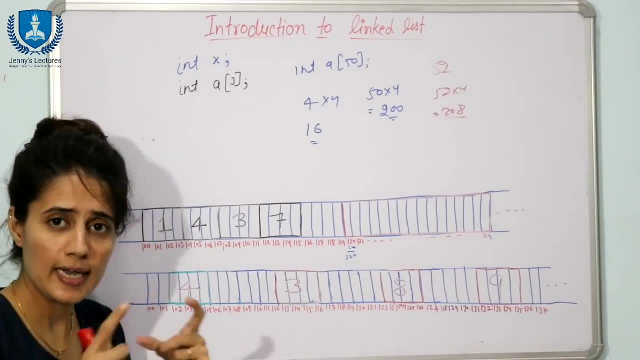 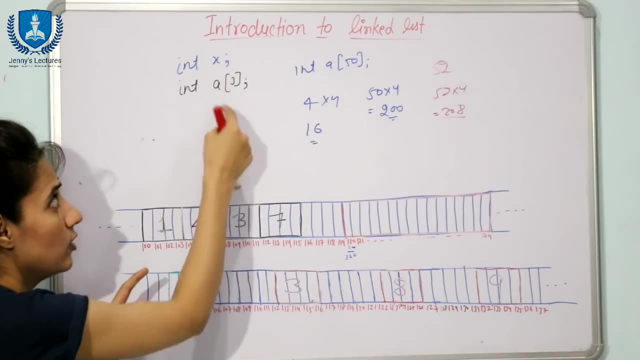 these four blocks to the programmer. so see here, these four values are also a collection, that is a linked list, because here i'm not discussing that he has. he has declared like this: int x, then int y, int z or int i, something like this: not variable, separate variables. this: 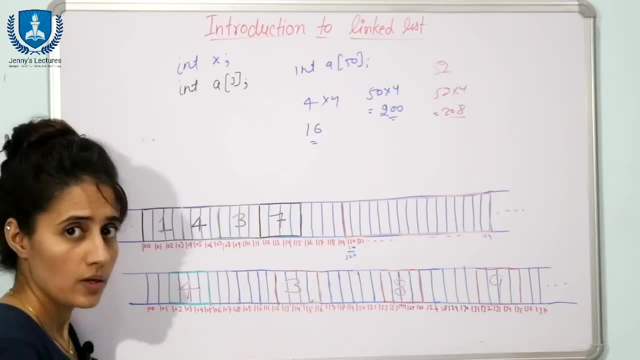 is also a collection. fine, this is also a list. now suppose if this, these four are in a collection, in array, that is fine, because these are consecutive locations. so if you know this thing, the base address of this one, you can easily, the compiler can easily compute this address of the next one. 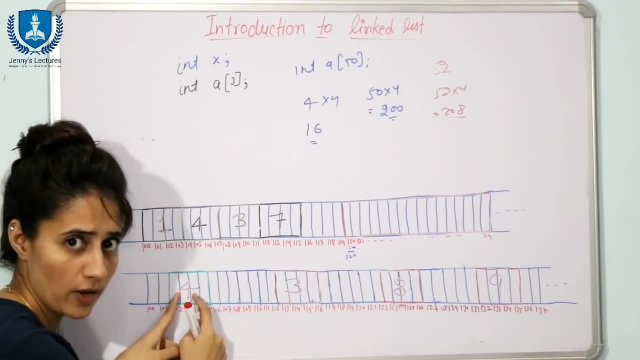 but here we cannot say: if this, we are at this value in this collection, if we are at this integer, then we cannot say at where, where the next integer is fine in that collection. so some extra information has to be stored. that is what if with the this thing, with this thing, with this? 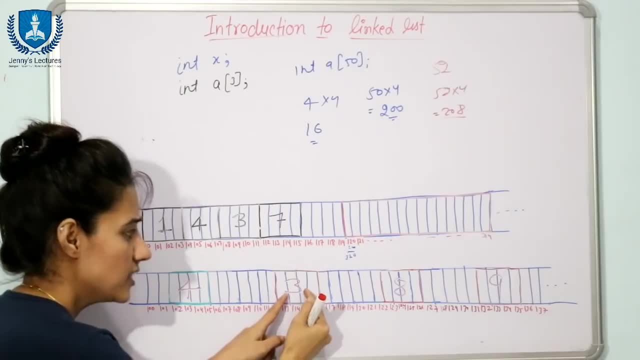 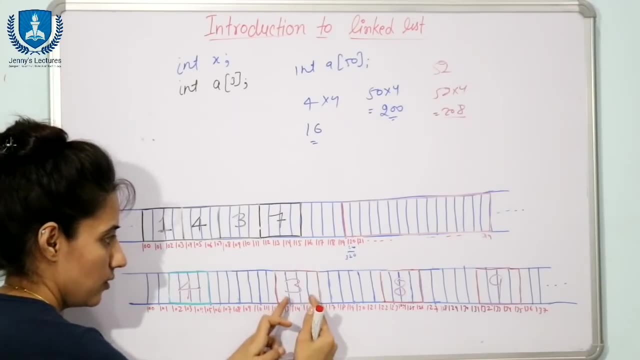 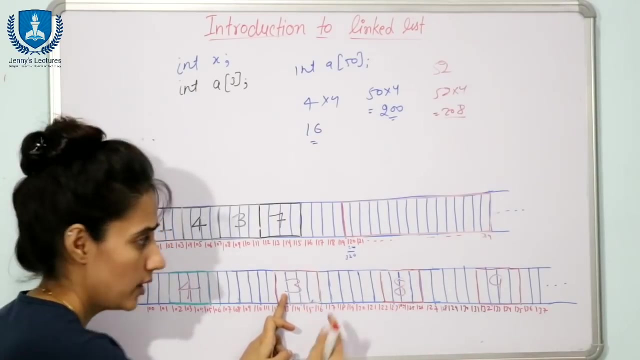 value. if we store address of that next value, then we can easily reach to here, fine, and from here in the list with this second value, if we store the address of the next value, the next integer value, then we can easily go from here to here and here we can store, with this value, the address of the. 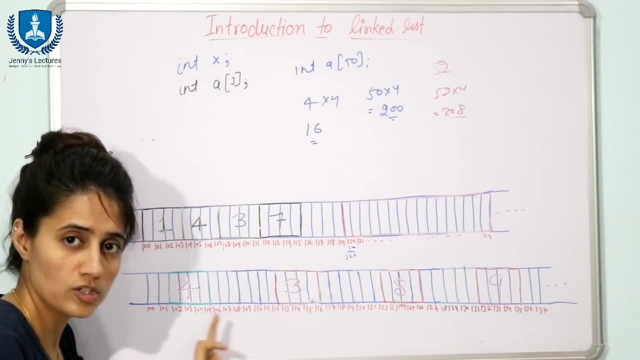 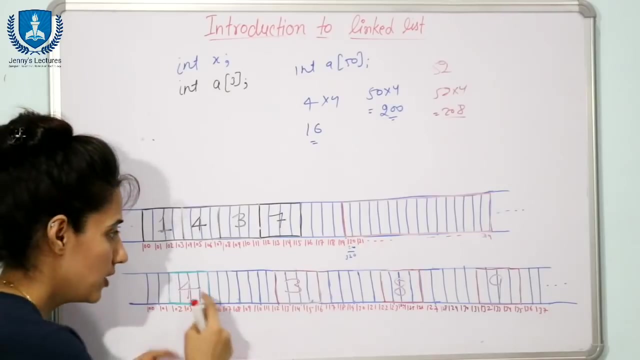 next value. fine, so this is what. this is also a collection of four integer values, but here the these values are not stored in contiguous location. we have removed that drawback. fine, now see. so some extra space is to be allocated with this one for storing address of the next value and address of the next value. which variable can store address of? 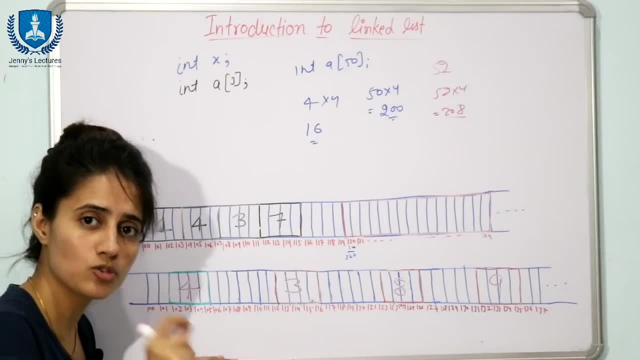 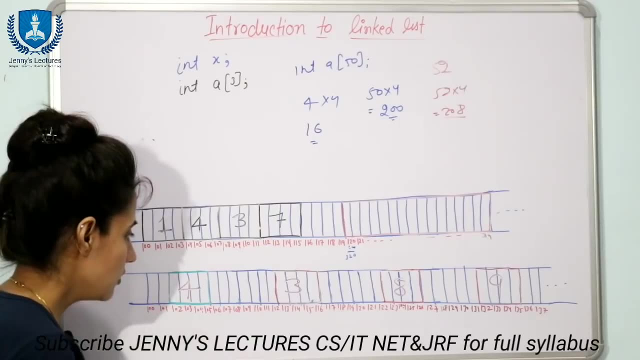 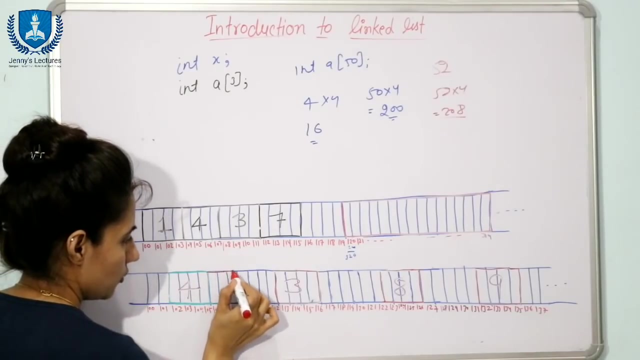 any another value, that is, a pointer variable, can store address of some another variable. fine, so here four bytes would be allocated again, because in typical compilers it the for storing the value, for storing the address, it takes four bytes. so see, here again four bytes would be allocated. 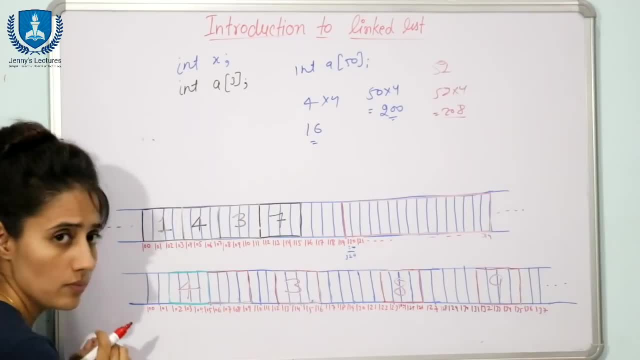 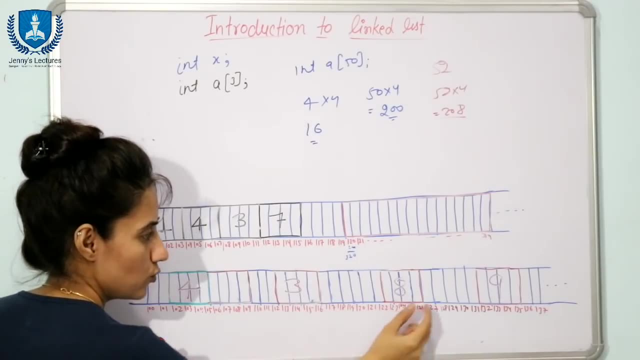 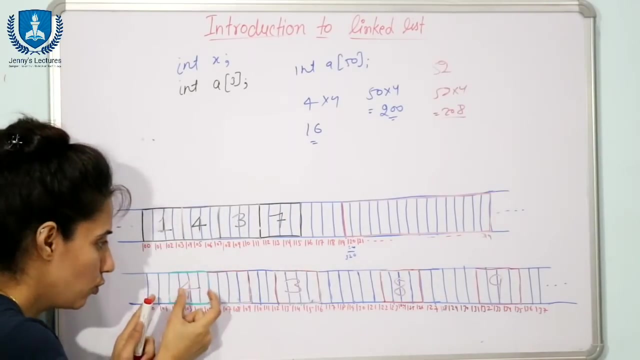 with this one. two, three and four fine for storing the address of this one right here, four bytes would be allocated for storing address of this one. here with this, four bytes would be allocated for storing this one. so, total, how many bytes would be allocated? eight bytes, four for this. 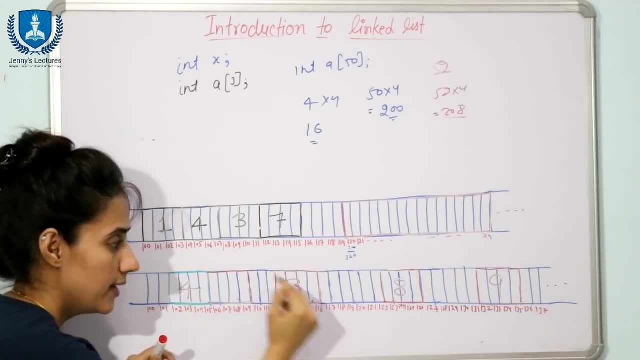 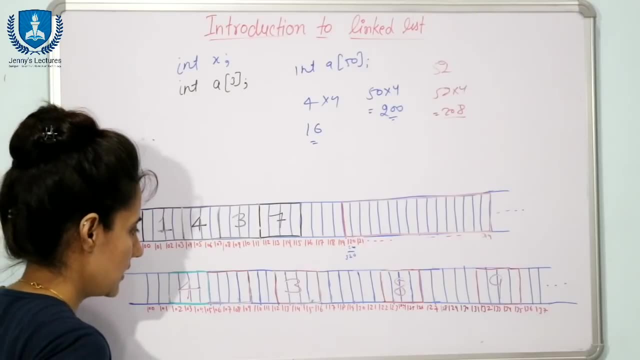 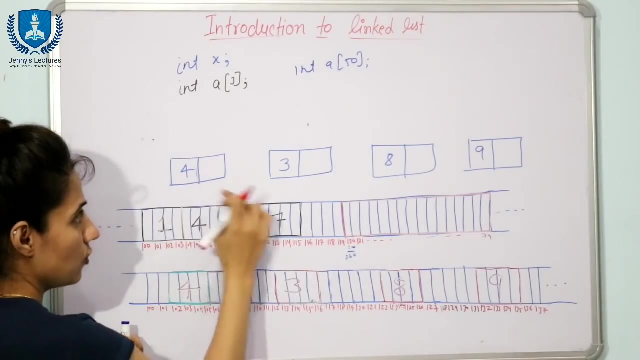 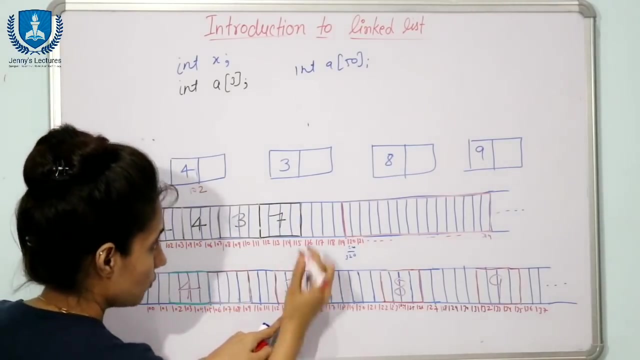 value and four bytes for storing the pointer to the next. well, right, so this is the memory representation. logically, how you will represent this link list: see four, three, four nodes: one is this, one, this, then this and this. with this four, address of next would be stored, see: suppose address of this is one zero, two for three addresses. we have started from one. 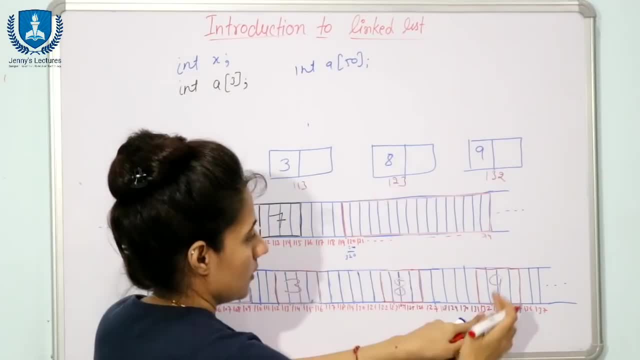 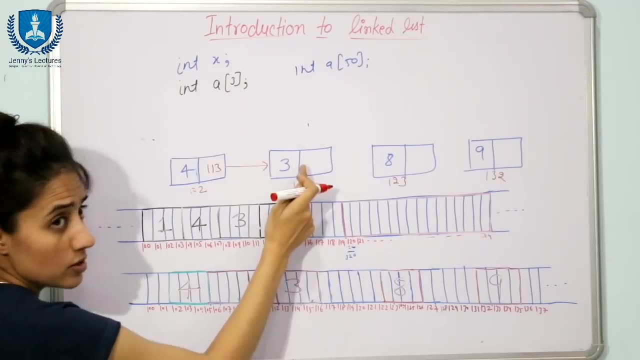 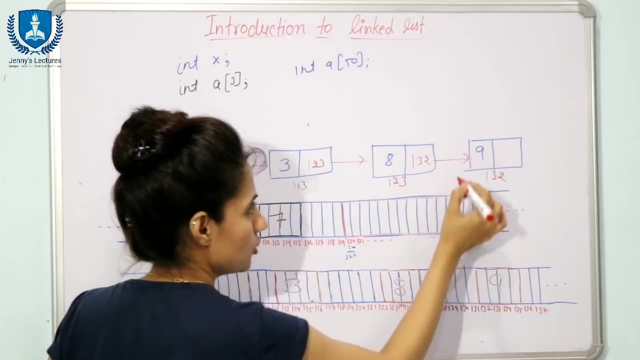 one three for eight. we have started from one two, three, and address of this is one thirty two, so here with this four, one one three would be stored, so this will point to the next node. here one twenty three would be sort, so this will point to this node. and here one thirty two will be sort. this will point to this nodes. 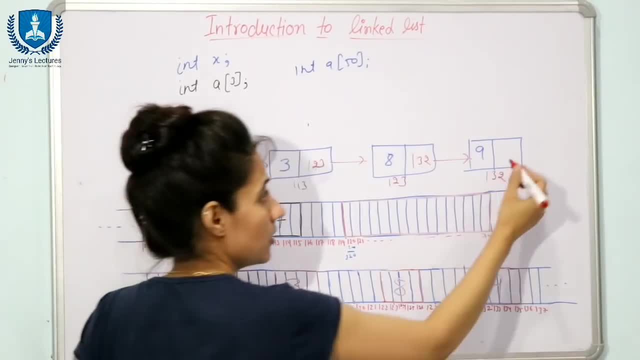 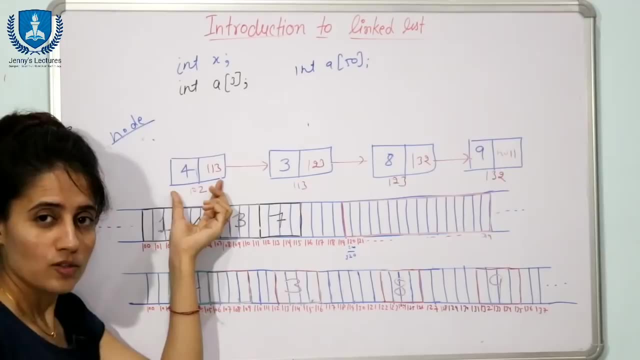 and suppose this is the last node in this list, so here now would be stored. so in the linked list this complete is known as a node. so here you can say: this is drawback of linked list with the. with this, well, you have a store pointer also, so some extra spaces to be a located the pointer to the. 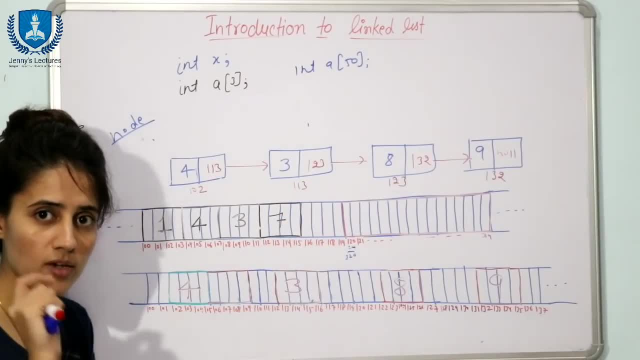 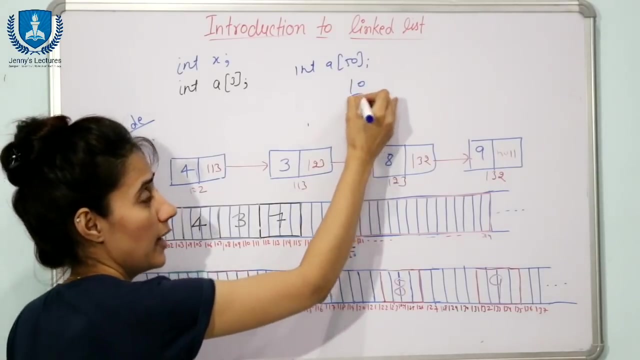 next node: video. another next node. this competes known as ap node here. fine, so this removes the drawback of array. now suppose i want to extend the size of linked list. i want to insert one extra element here. i want to insert 10 in the in my linked list. 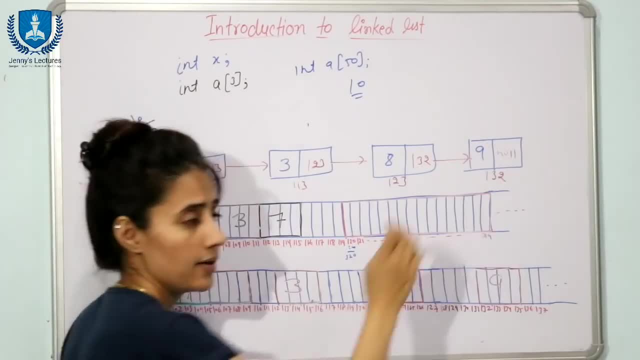 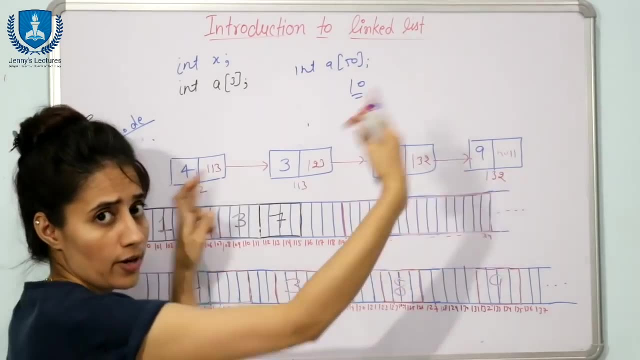 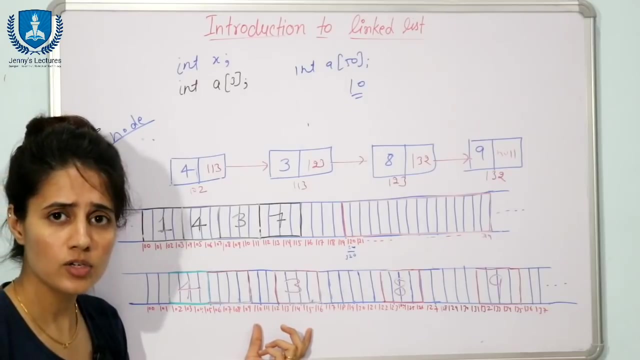 right now, suppose i want to insert 10 here. so here can we insert this 10 directly here, or the memory manager will allocate space for all the five variables. some fresh block would be allocated. no, why so? because these values are not not in contiguous locations. so if anywhere space is, 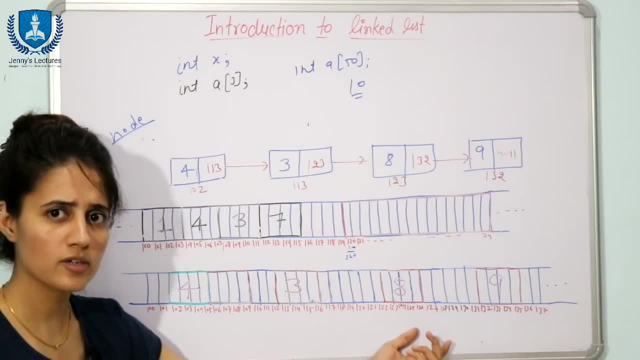 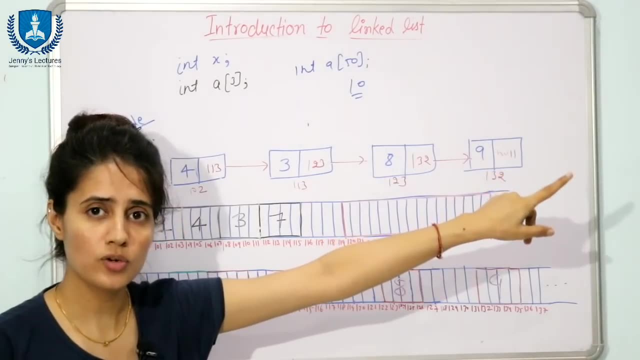 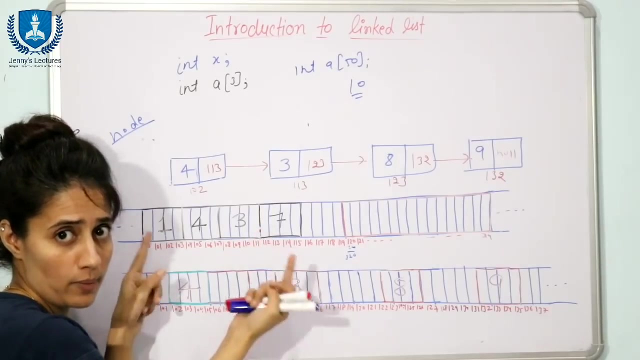 available for eight bytes, then memory manager can allocate space there only fine, and we can provide link to link into this node for that new node inserted. but in array we cannot do this because in array drawback is what all the value should be in consecutive locations fine. so maybe sometimes. 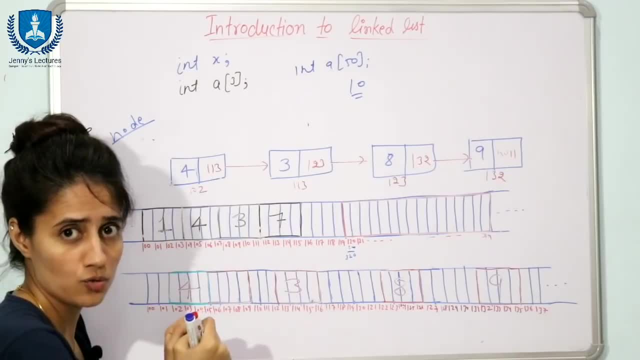 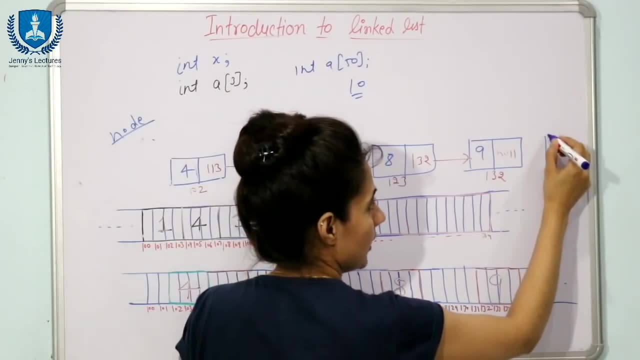 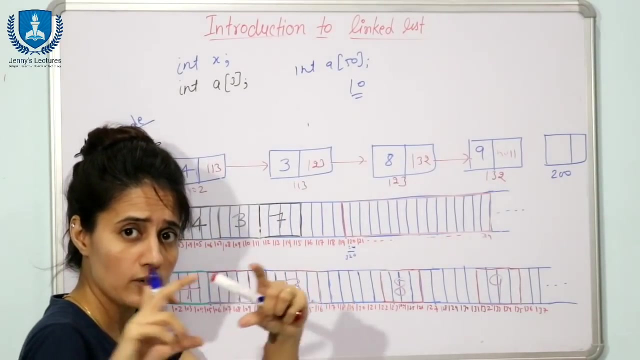 it is not possible to extend this size in case of a, a. now, if you want to insert this 10, so simply somewhere in memory. somewhere in memory, suppose address is 200 and node is to be allocated, a memory size of 8 bytes is to be allocated. that 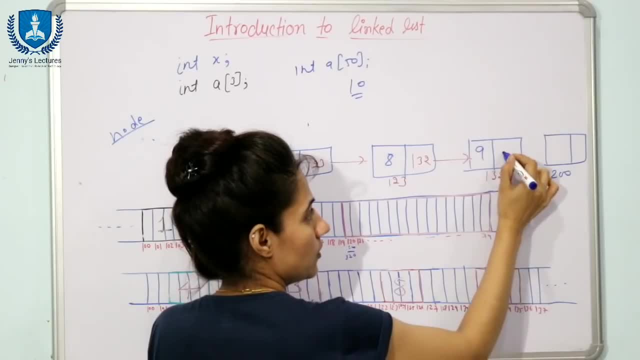 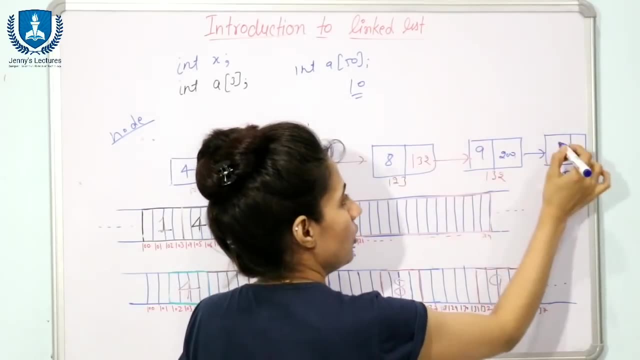 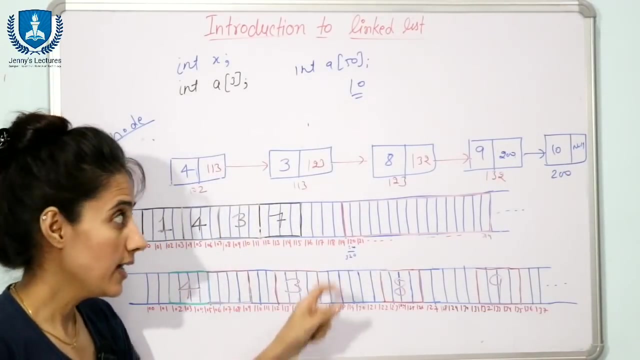 is known as node, and here this 200 would be stored in the link in the pointer part of this previous node. fine, and here the value is 10, and if this is the last one, so here you can store none. so this is how you can see that insertion in a linked list is very easy. thank god we. 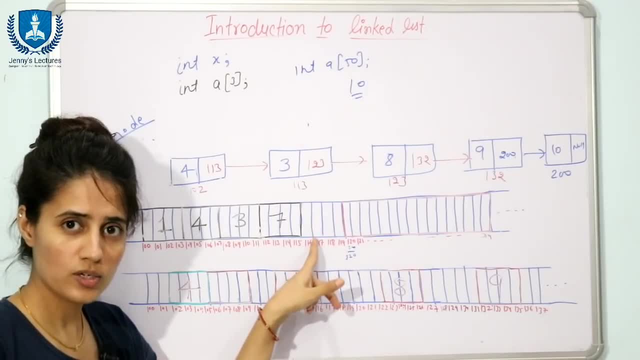 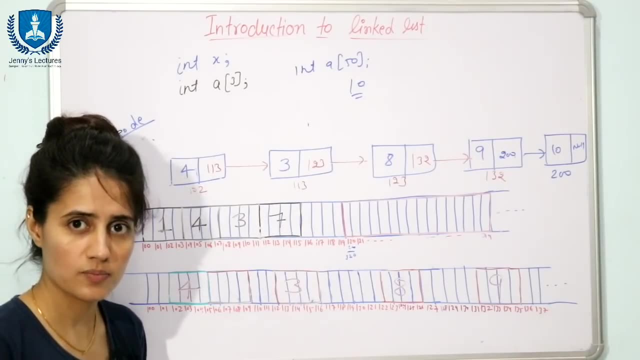 can see. we have removed that fixed size drawback that was in array. no need to specify the size. that in the linked list. i want 10 elements, 20, any elements like this. you can insert any type an element from in the linked list so when you write a program. 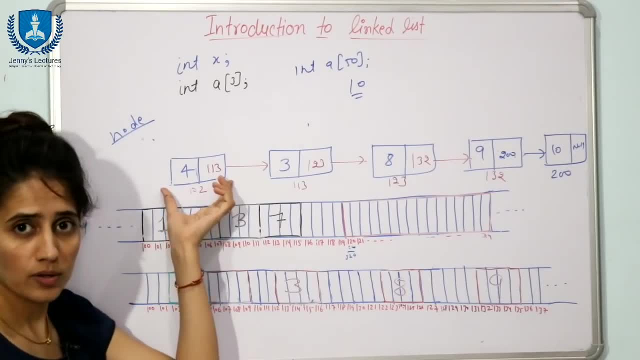 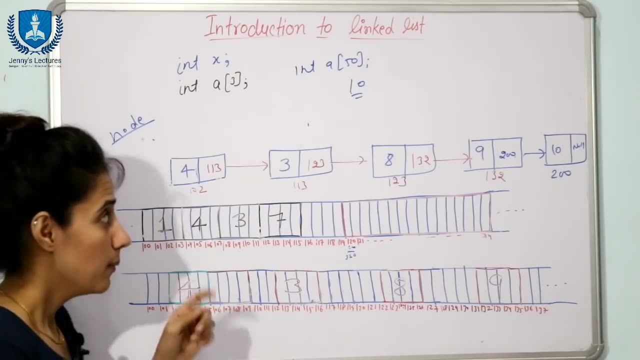 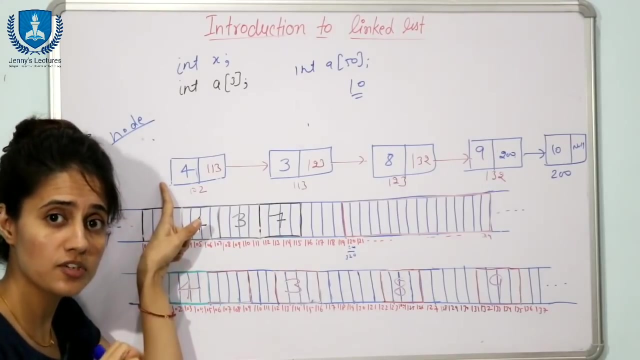 in linked list, then how you will declare this node in array. if you want to declare simply, you will write data type, array name and size. that is very easy. but in case of linked list, see this here: this particular node is containing two values and type of two values is different. one is integer value. 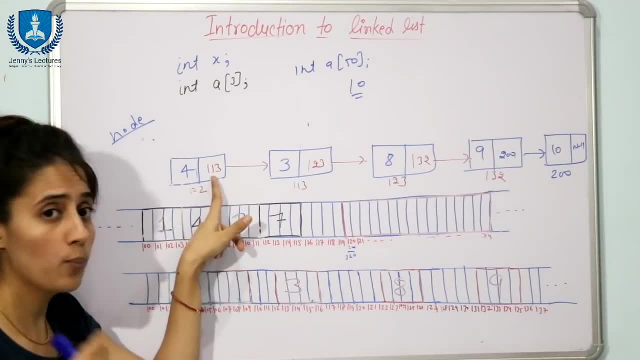 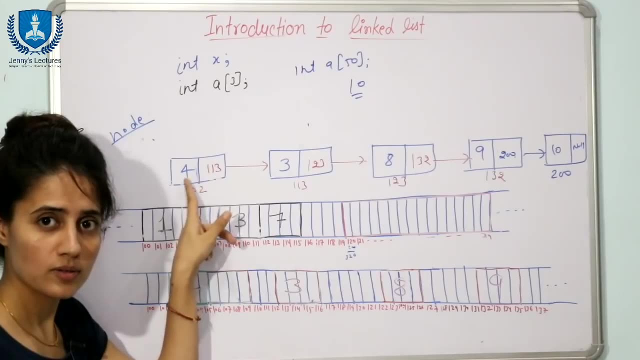 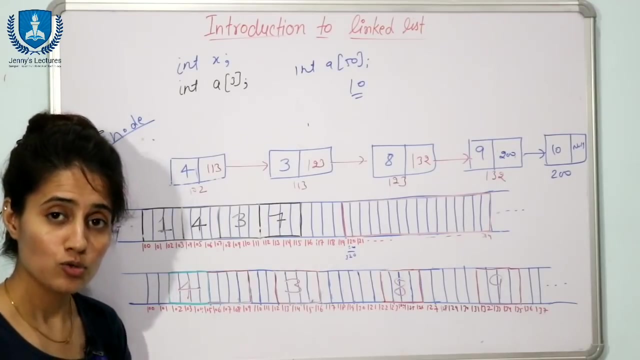 and this one is what address. so this is what a pointer, not a simple variable. this is simple variable. this is what a pointer. two types in one node- fine, so you have to define your own data type. fine, so that user defined data types you are going to use. that is structure, so you are going to write. struct. so after this struct keyword you are going to give the name of your data type you want to create. fine, here i'm taking the name node, struct, node. so within this you will write: see. want to value. the type of 1 is integer, so here you will write. 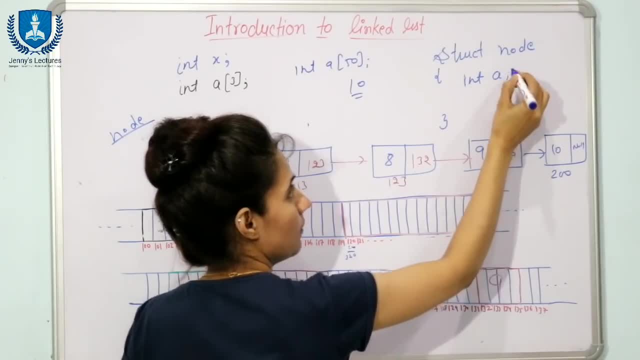 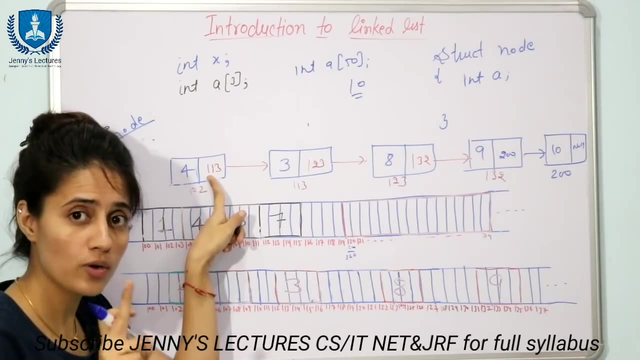 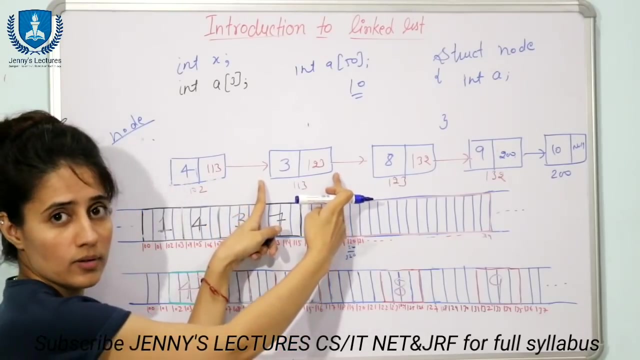 int. suppose a name of variable is a, but this is what for this, how you will declares is a pointer, because only pointer can store address of another variable. and this pointer is going to store address of this node, right, not address of any other variable or any other. 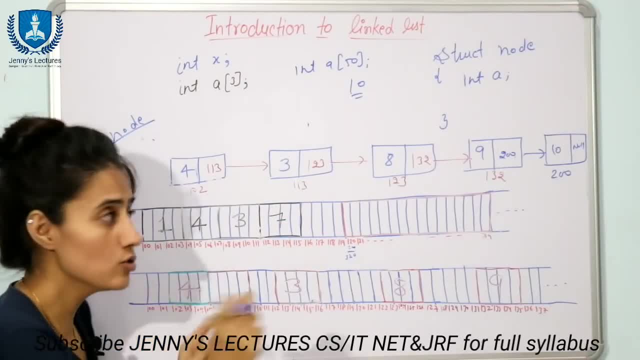 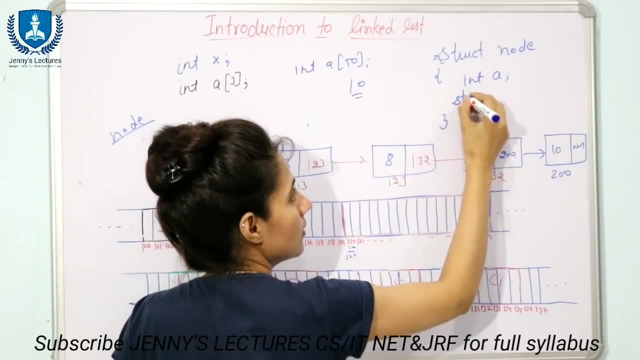 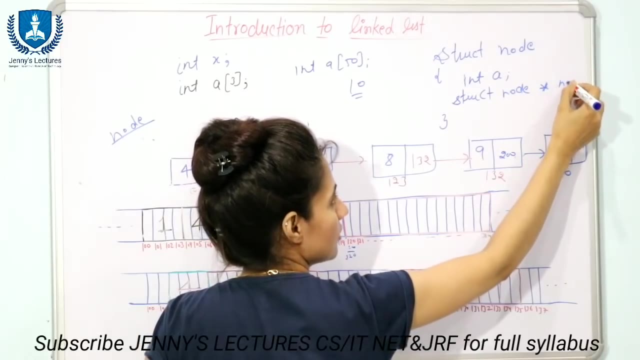 integer variable. by the way, sometimes, if you have x in solid, that is not the case, but 종 we can. this pointer is going to store address of another node. fine, so here you will write what struct, node, pointer and name of the pointer you can say next. so this is how we are going to define. 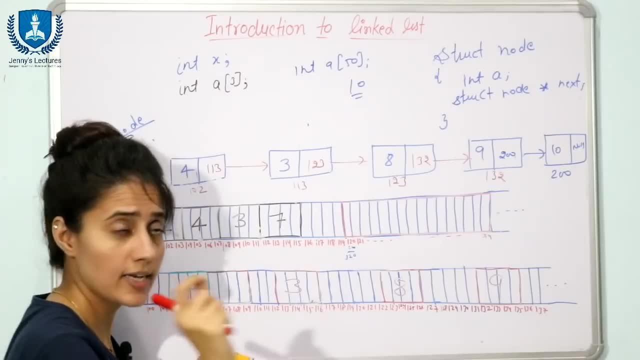 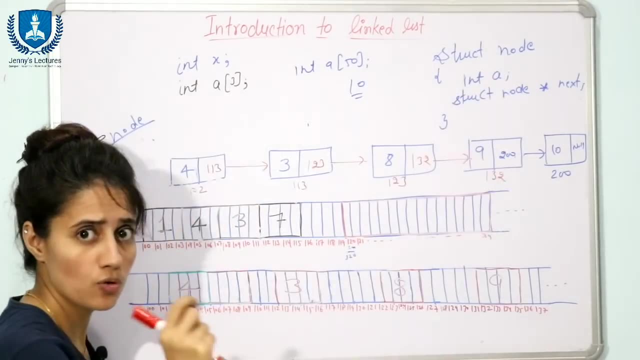 our new data type, that is struct node. the name of the data type is complete. this one struct node, not only, not only node, that is struct node and these are members of this structure. here you write struct keyword, then tag, and within this you will write members. ma'am, two members are there one? 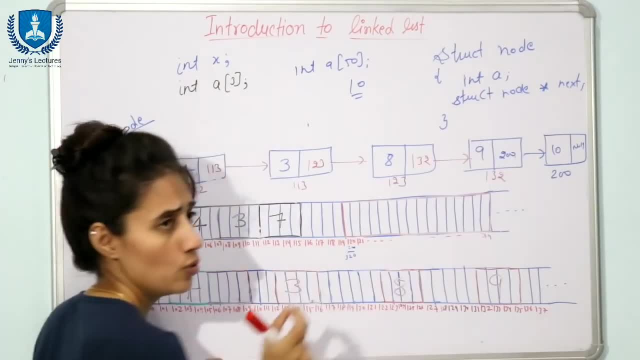 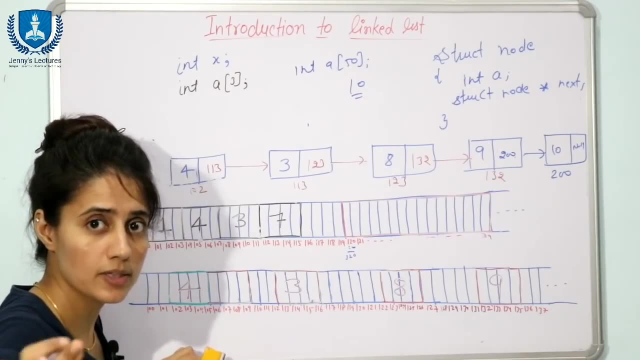 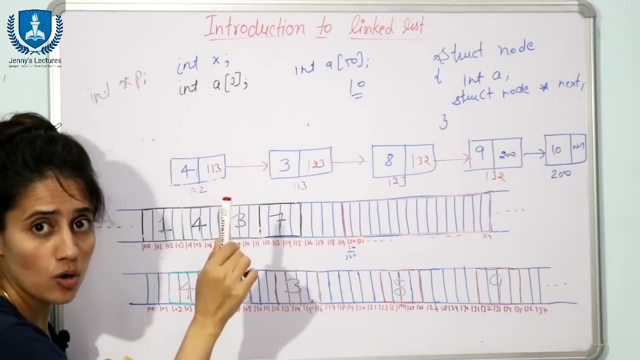 is this one one. is this one now why i am writing here struct node. as you know, if you want to declare a pointer which is going to store address of some another integer variable, then how you will declare int star p. this p is going to store address of integer. 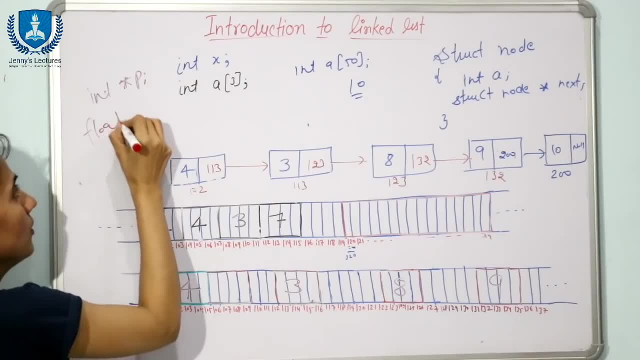 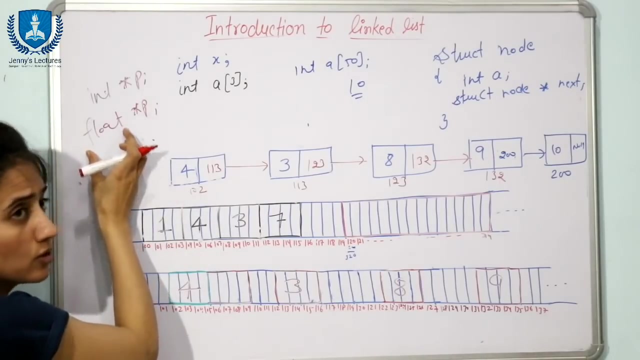 variable. fine, if i write float asterisk p, it means this p is going to store address of a float variable. it means it is pointer to float, pointer to int. so here this is data type. this data type is what this data type is for the variable whose address this pointer is going to. 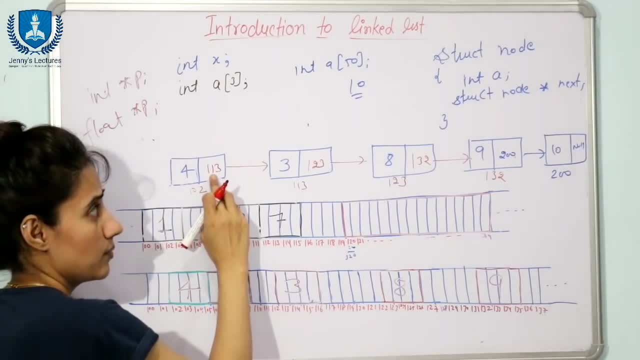 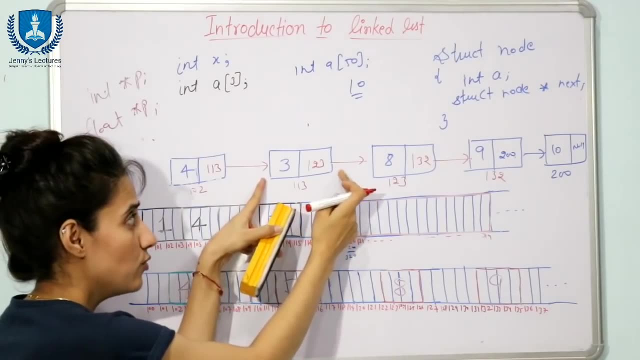 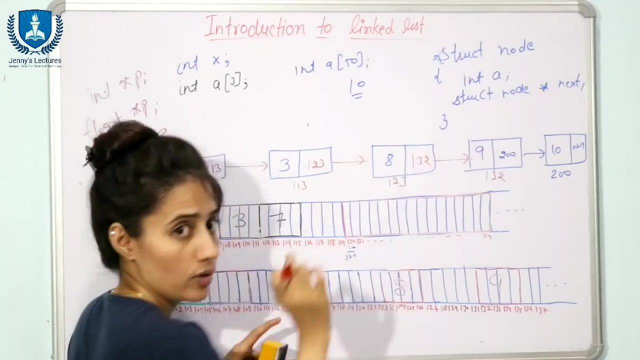 store. fine, now here, this is the pointer. the pointer is going to store address of this one, this one: this is what node and data type of this node is what this complete struct node name of data type. see, this is data type struct node. so that is why here i am writing data type. that is struct node. this is: 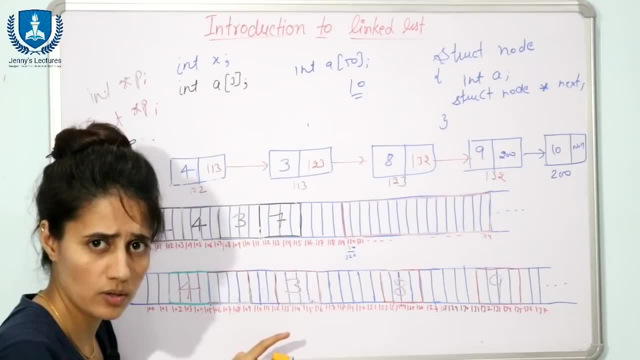 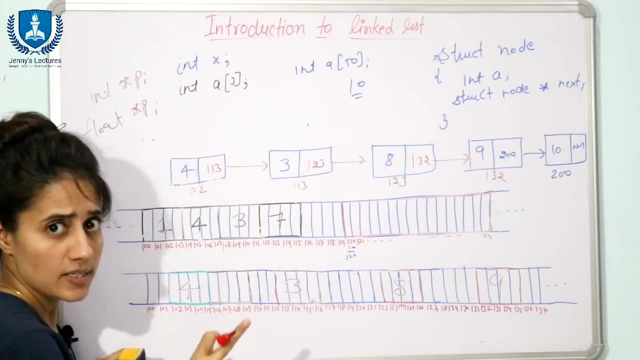 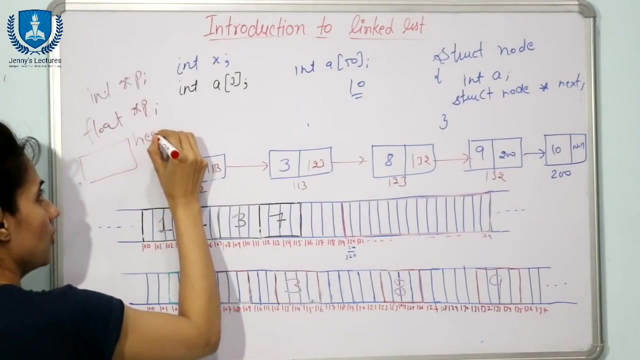 same asterisk and this is pointer name you can write next you can write your here link. it's up to you. fine, now next thing is: this is the link list. now another pointer is there. you can say head pointer, start pointer, it it's up to you. this pointer is going to store address of the first node in the. 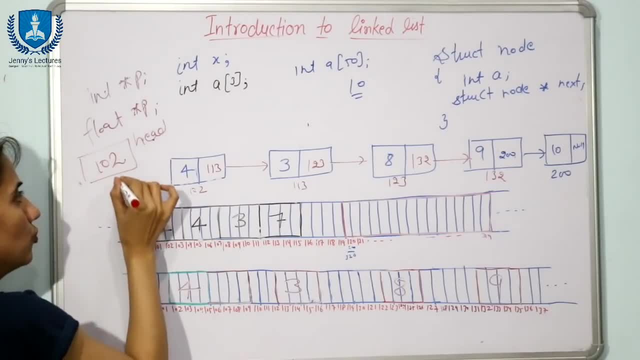 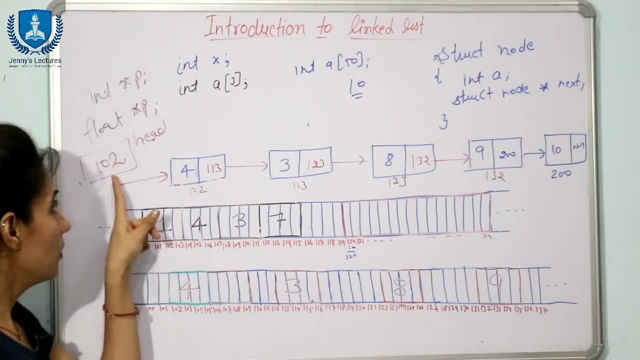 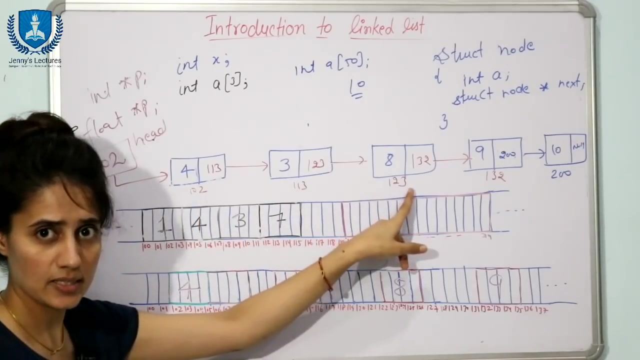 link list address of first node is 102. so this head is going to point to the first node in the link list, right? if you know this, this address 102. if you know the value of this head, this pointer, then you can easily traverse this link list. fine. but here random access is not possible in array. 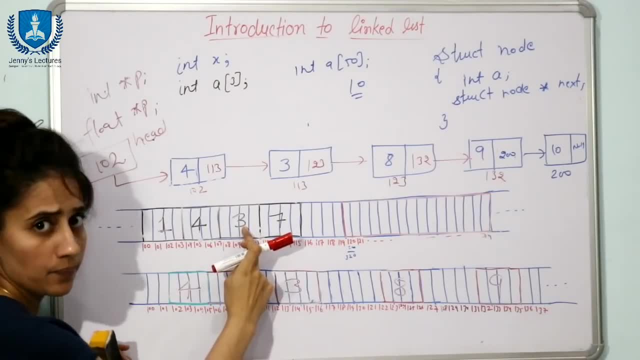 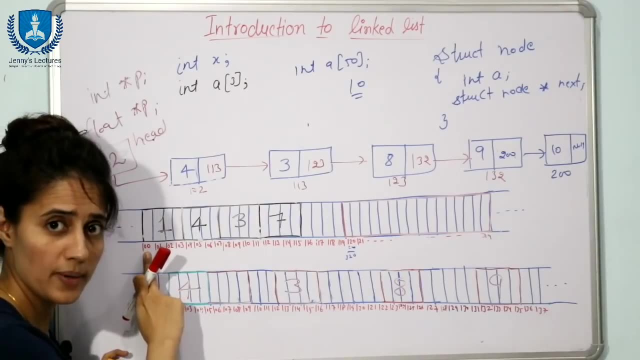 what is there. you can directly go through this and you can easily go through this link list. if you want to access this three, you can directly access this three. compiler can directly compute the address of this three if the compiler know the base address. but here, if you know the base, 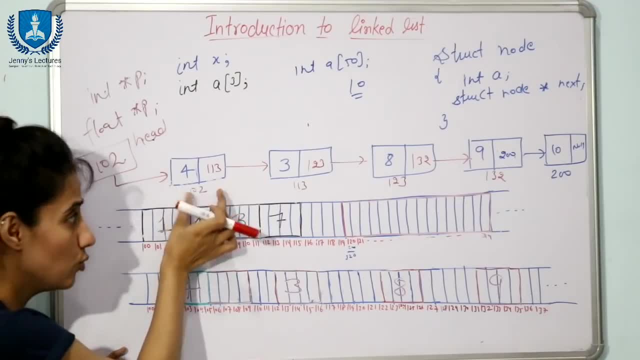 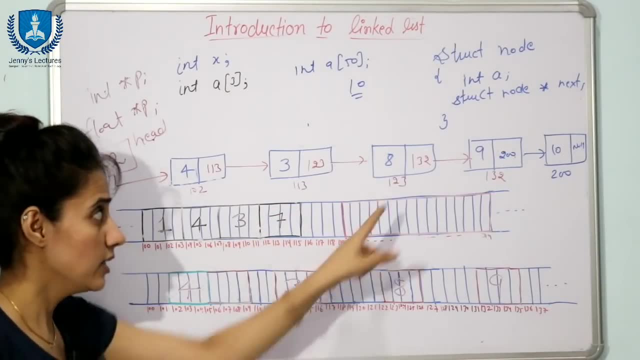 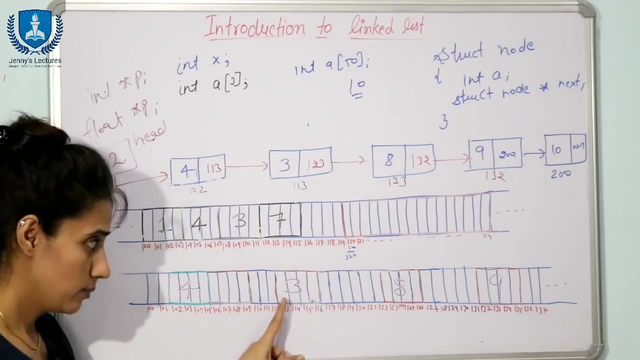 address. that is the address of this first, first node. that is one zero two. and if you want to access this one, this node, this data, you want to access, but you cannot directly go here. compiler cannot directly compute this address. fine, that is drawback of this thing, because her that data is. 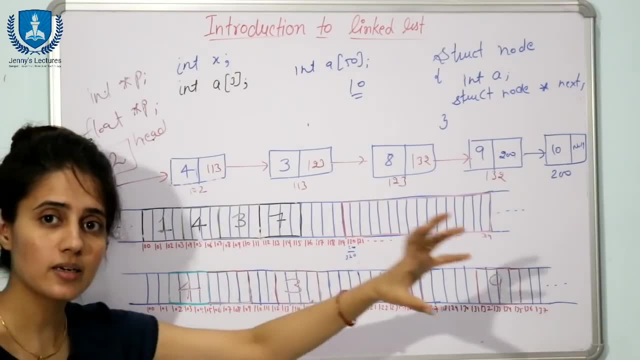 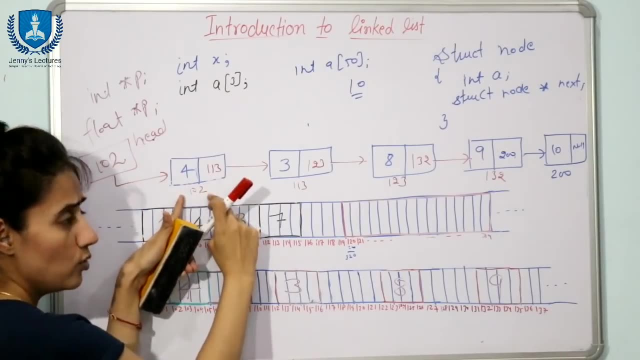 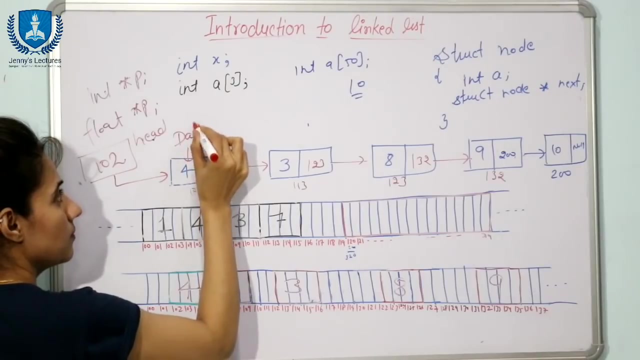 not in consecutive locations, it is in scattered locations. fine, so if you know this value of this head, 1 0, 2- so here you can go, from this node you can go where check out the link part. see, this is what data part and this is link part of the node. fine, so check out the link part and 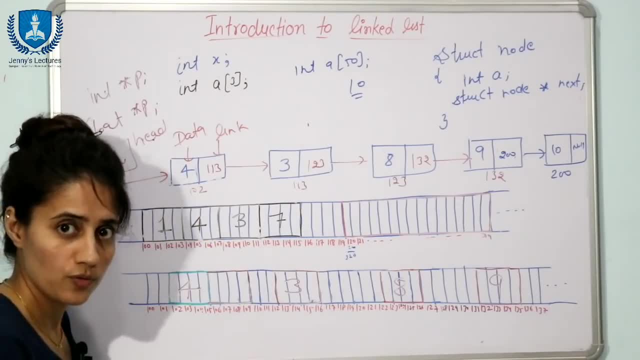 there is the header in address ninety zero two and so this is just eramto. from search select the location of the linked on the SPD data link link part here, the address, address of which node 113. it means address of this node, so you can go. 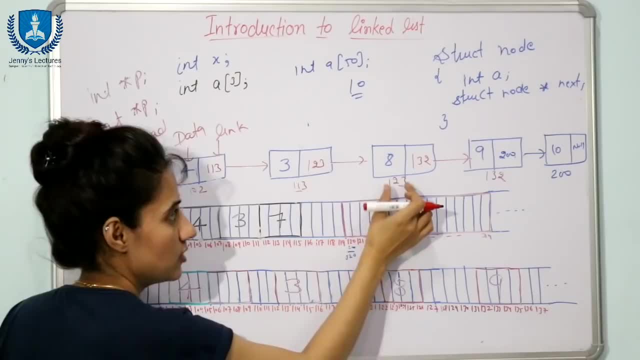 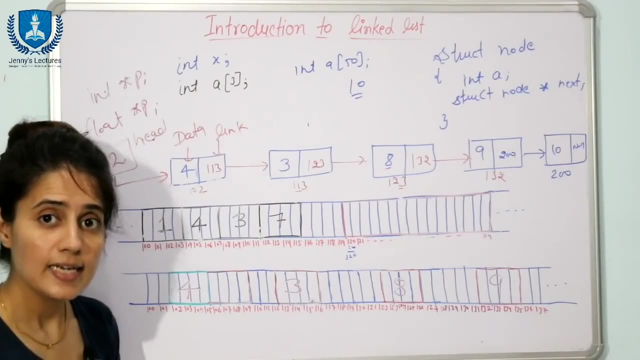 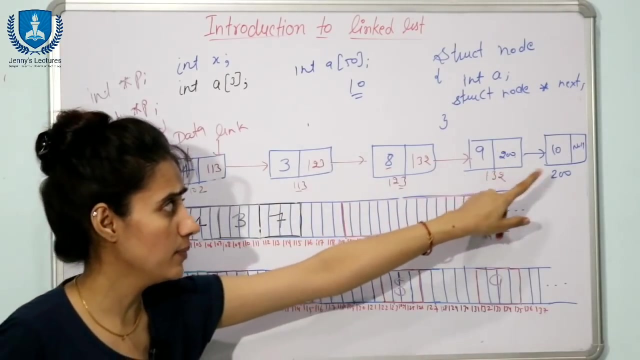 to this node. now check out the link part one, two, three here address is this one. you can go to here. one, two, three, so now you can reach here. fine, so in link list only sequential access is possible. you cannot directly access, you cannot randomly access any data. fine, if you want to access this. 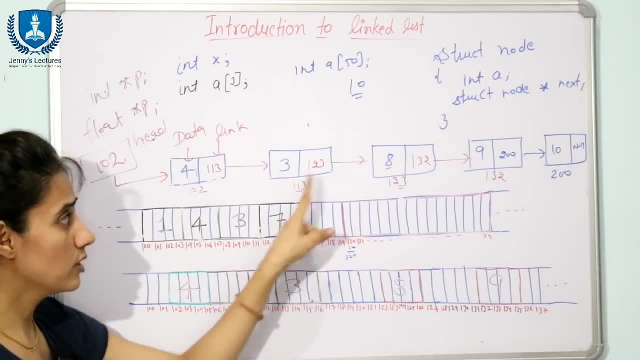 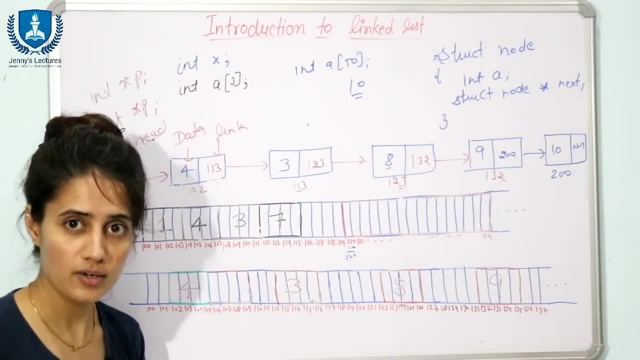 last data. then also you have to traverse the complete list, first of all this, then this, then this, after 1, 3, 2 and after that you can go here. fine, so this is, you can say, a drawback of this thing. so this traversal need, or you can say this: searching will need the time, complexity, the time. 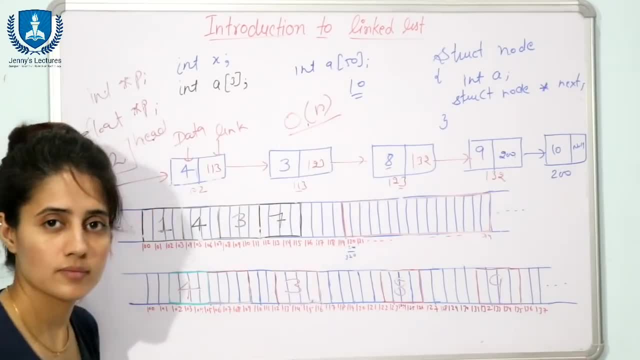 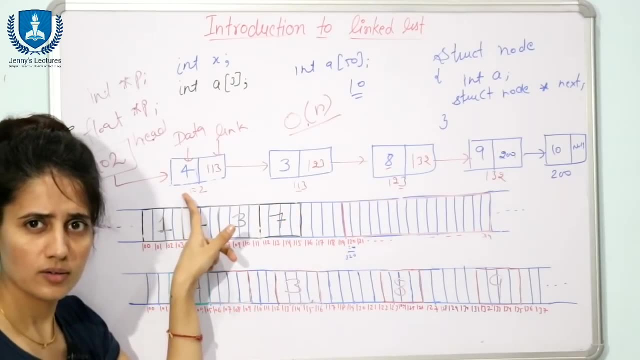 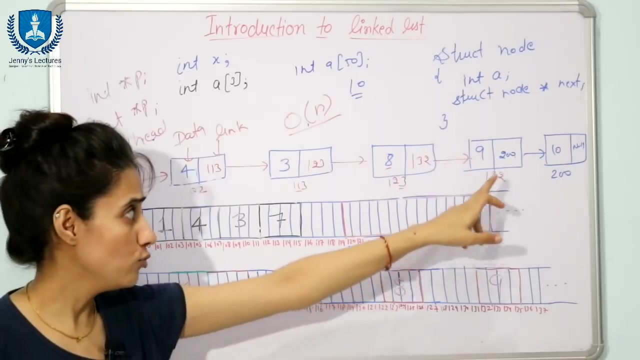 is order of n. accessing of any elements need order of n. in worst case if you want to access the first element, then obviously it is one, only order of one. if last means in worst case it is n, you have to traverse the un? n elements in the list. so it is order of n, but in array it was accessing of. 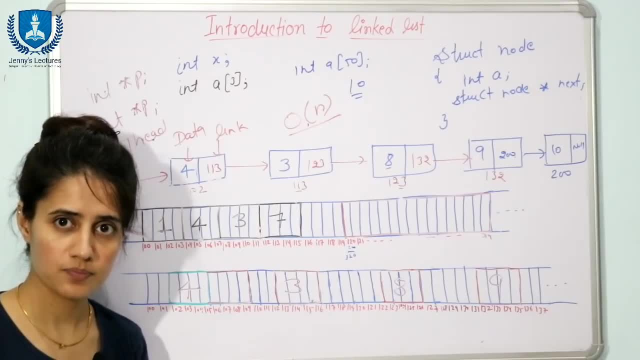 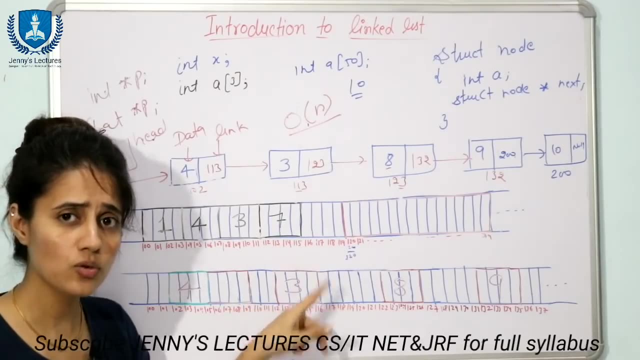 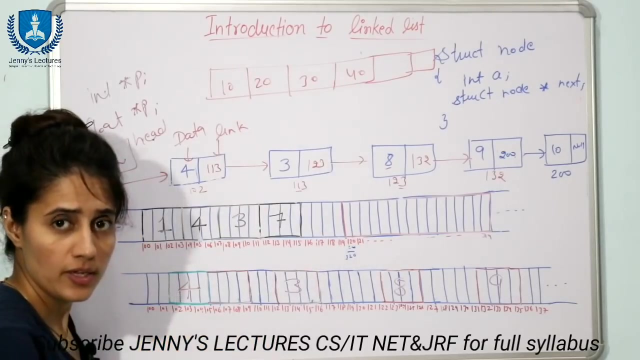 any elements will take order of one only constant time. fine, but here insertion is easy and deletion is also easy. why so? because, see, if sorted array is there like this: see, let us take an array of size 6. only 4 elements we have in the array and i want to insert 5 here. this is sorted array now where 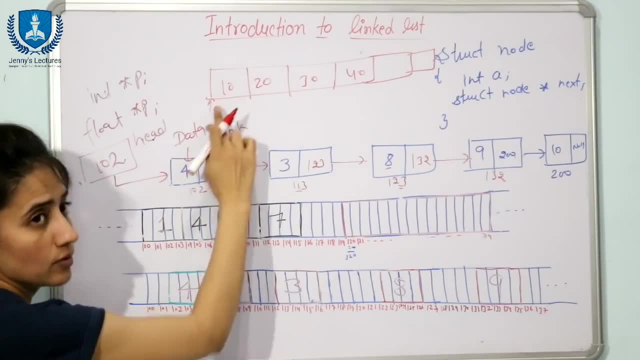 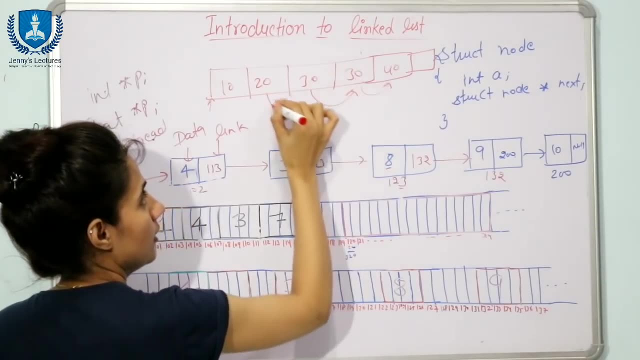 you can insert 5 here you can insert 5, only fine. so you have to do what you have to shift this 40 here. here you have to shift 30, here you have to shift 20. here you have to shift 10 and here now. 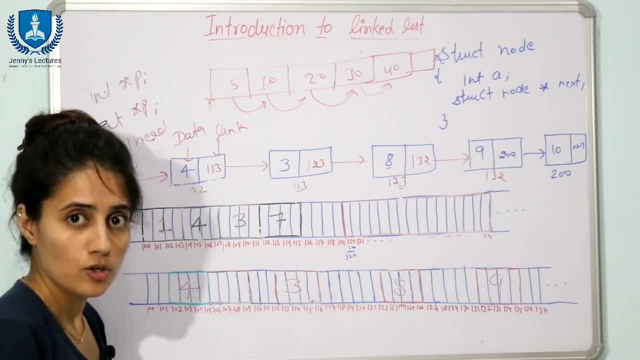 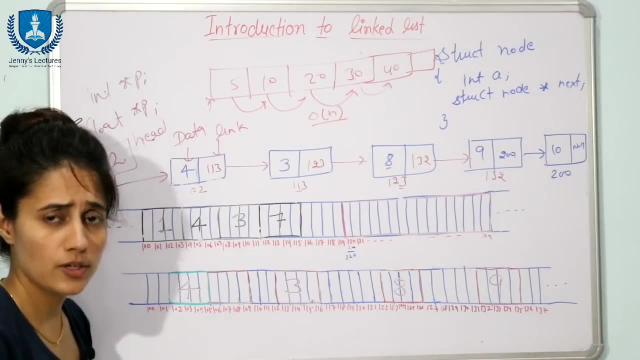 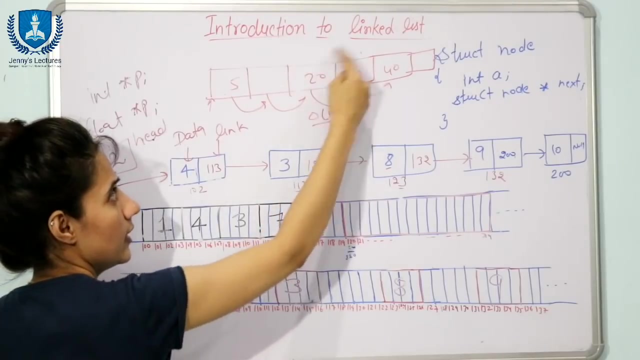 you can insert 5, right, so it will take how many shifting of all the elements. so order of n. if you want to delete- if suppose i want to delete this 10, i want to delete this 10- then also you have to shift 20 here, 30 here and 40 here. then also it is approximately you are going to take. 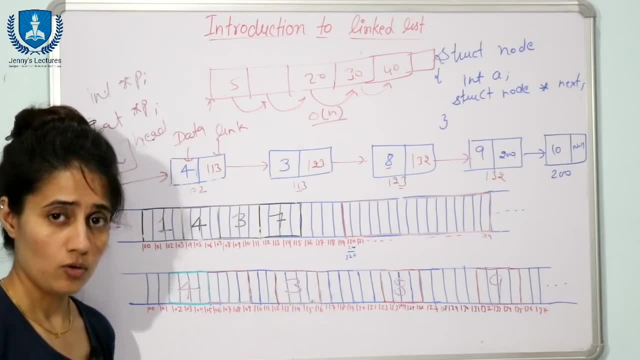 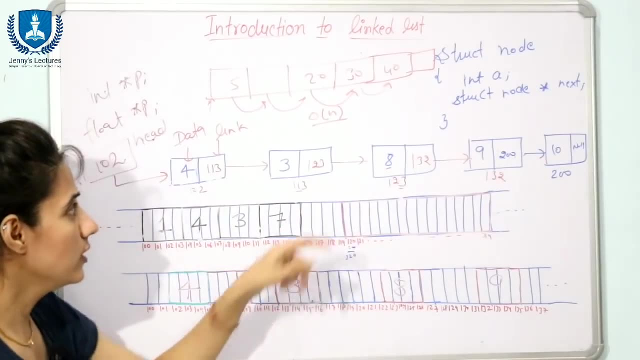 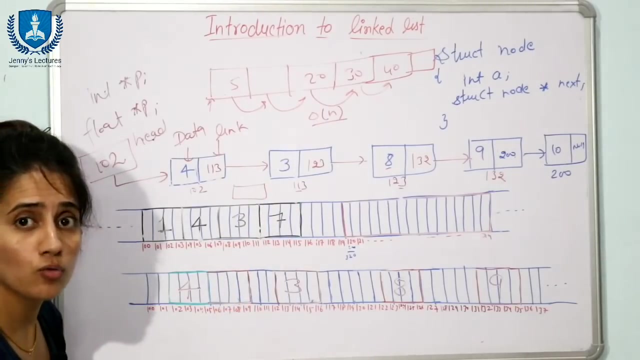 order of n. fine, or it depends the position from where you want to delete and at which position you want to insert the data. right, if you want to insert, suppose between these elements right here one node i want to insert, then what you have to update, just you have to insert the data. 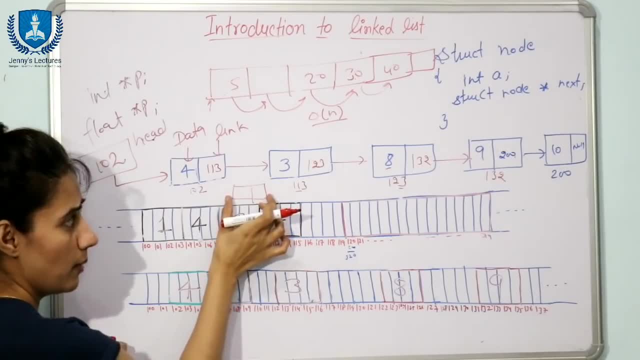 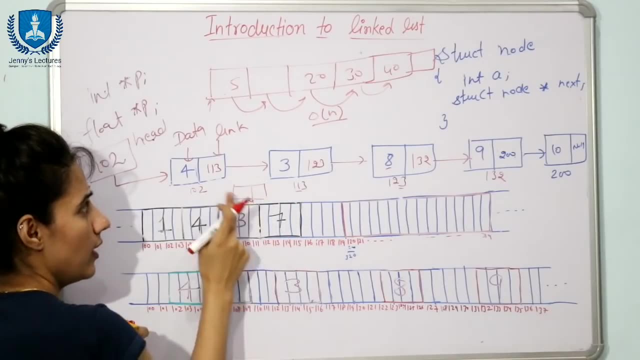 on that direction, because society hate this space again. so this integration again. this is the way how you have to update. see suppose, address this: this memory location has been allocated here. suppose that the 300 at 300. fine, so what you have to do: this 300 should. 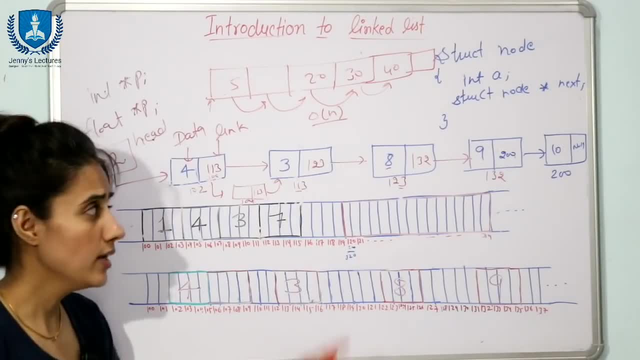 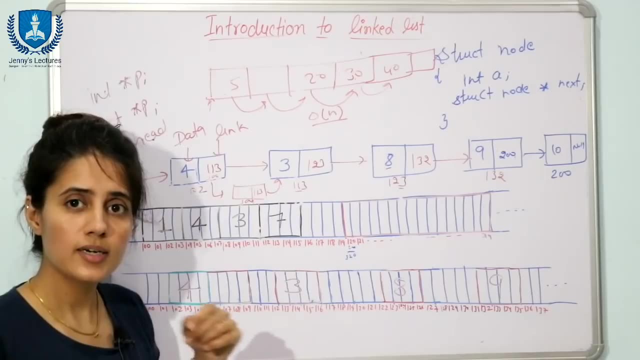 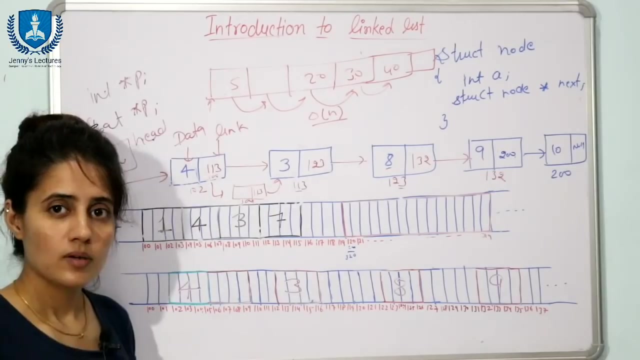 be here and this one one, three should be here. so this link would be something like this: as simple as that, right? so insertion and deletion is easy in this case, rather thanAray. so briefly, you say data elements which are stored in known consecutive locations. next point is some. 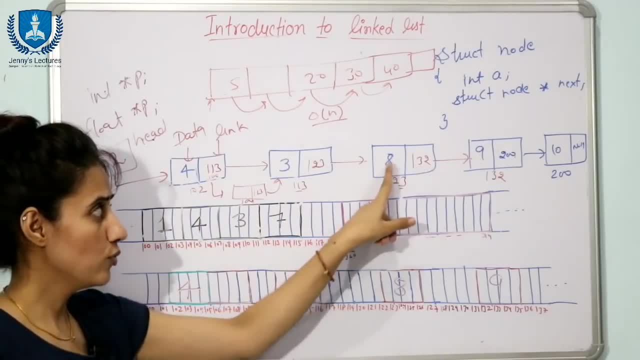 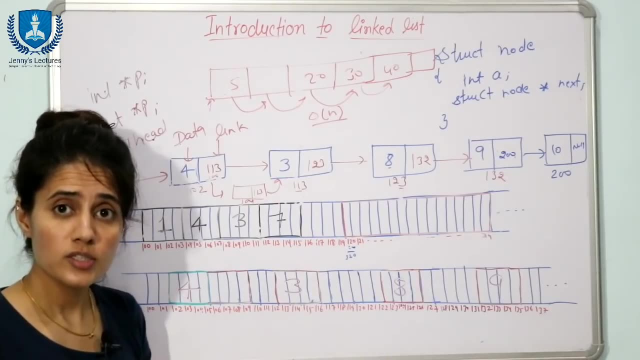 extra space would be required to store the pointers with each value. next point: you can say: insertion and deletion is easier than array. next point: you can say: accessing of any element is going to take order of n time complexity and in array it is order of one only. next point: you: 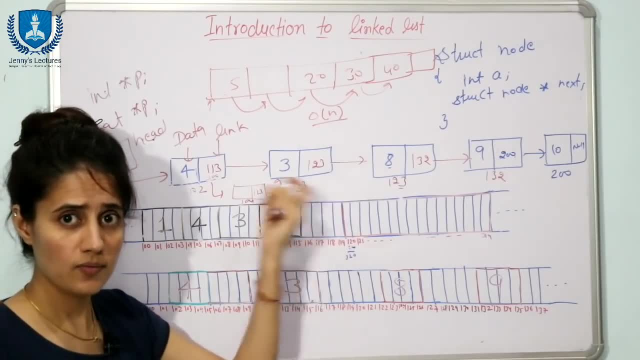 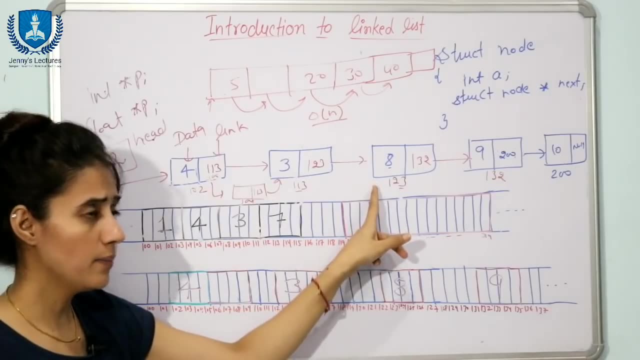 can say: binary search is not possible in linked list, in this fundamental, this structure of linked list, because binary search in that case you have to find out middle element. so here we cannot go directly to middle element. so you can say binary search is not possible. next point: you can say it: 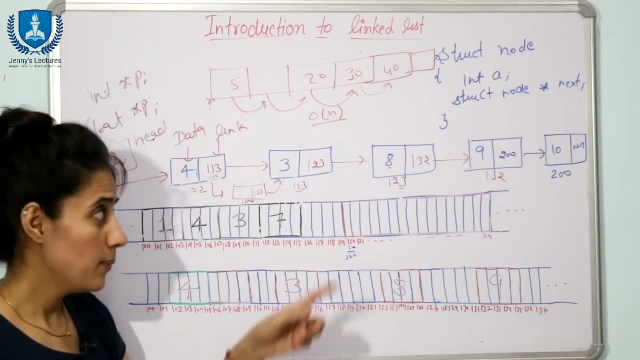 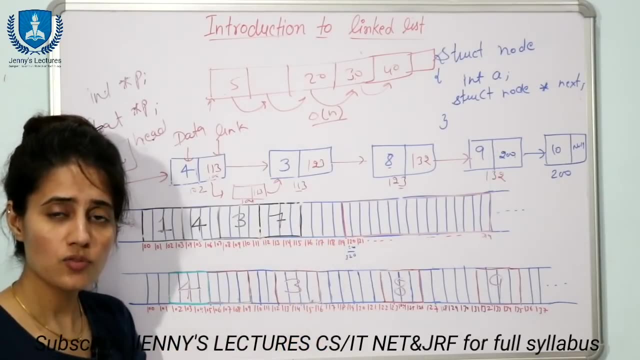 is of dynamic size. so in next video i'm going to discuss the basic operations of this linked list: traversal, insertion, deletion, something like this- with the help of their code as well, as we are going to discuss types of linked list. fine, so i'll see in the next video. till then, bye, bye, take.